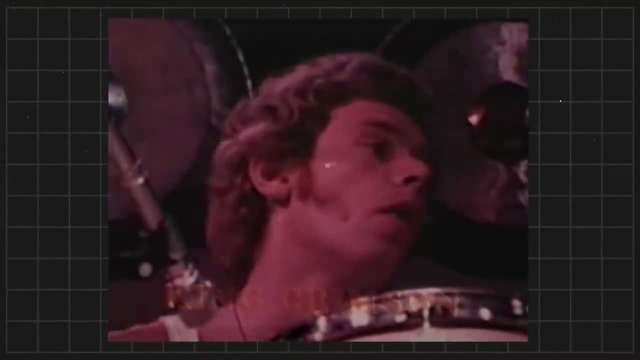 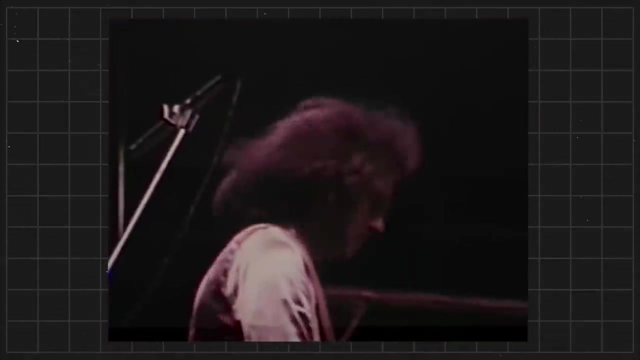 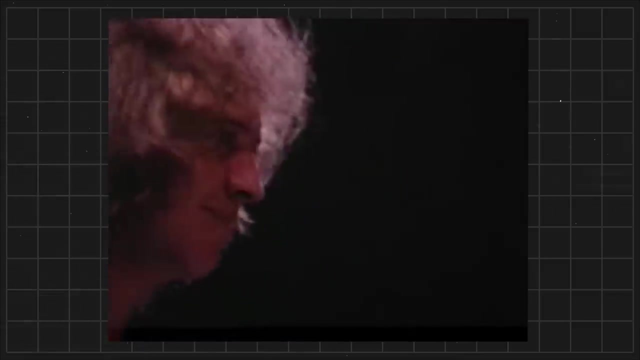 King Crimson is one of the most important bands in the history of music. It has not achieved the household name status or multi-platinum sales of acts like The Beatles or Pink Floyd, but it pioneered a new genre of music and has repeatedly broken new musical ground. 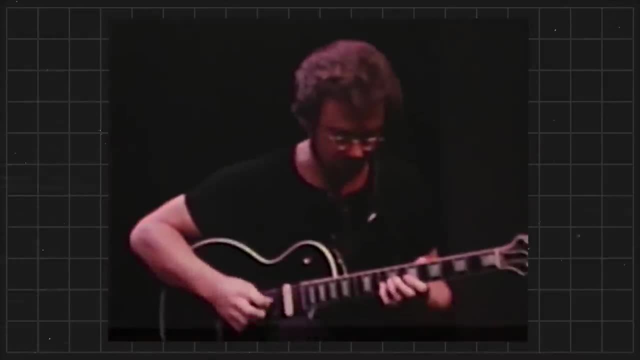 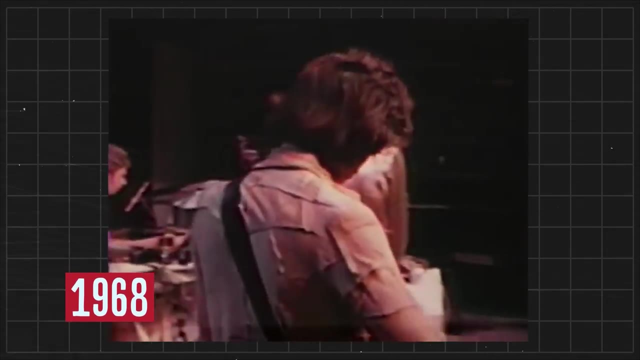 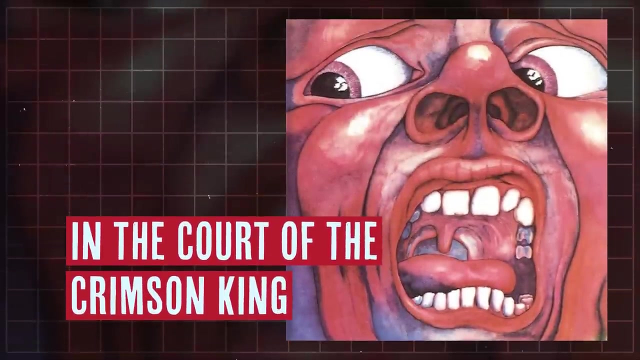 And every single one of King Crimson's musical innovations has been hugely influential on a wide range of bands and artists. King Crimson was founded in 1968 and laid the foundation for the prog rock genre with its debut album In the Court of the Crimson King, which also contained prototype heavy metal. 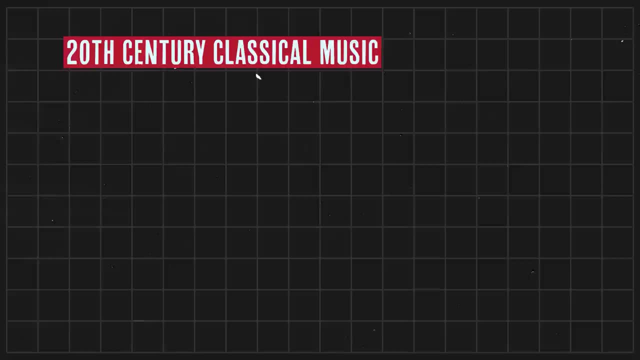 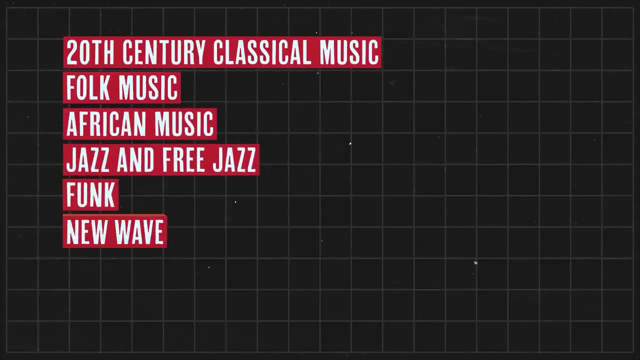 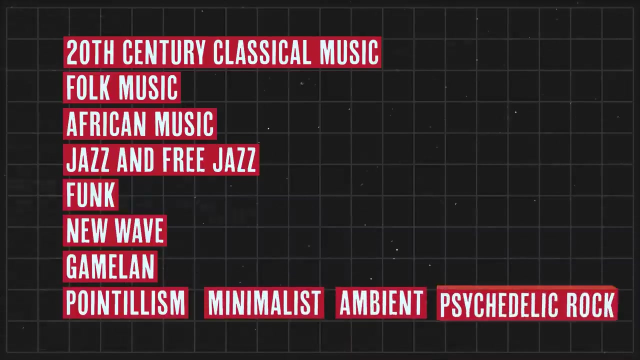 King Crimson has since incorporated influences from 20th century classical music, folk music, African music, jazz and free jazz, funk, new wave gamelan, pointillism, minimalist, ambient, psychedelic rock, industrial music, electronica and even drum and bass and techno. 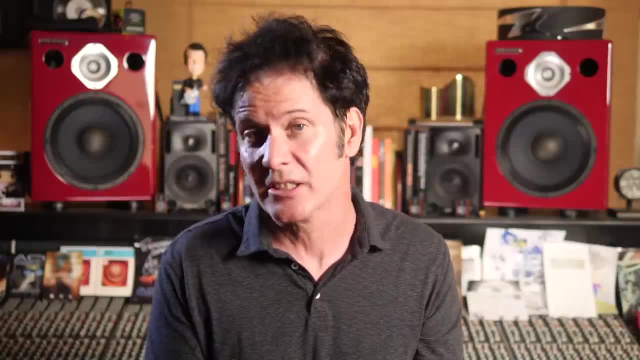 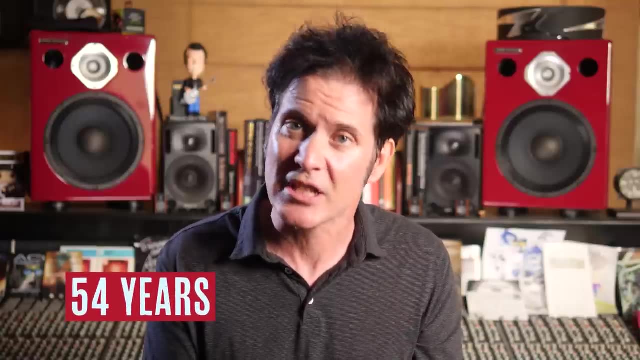 One thing that sets the band apart is that it is not significantly influenced by blues. King Crimson is still in existence today. In the 54 years since its inception, the band has gone through countless personnel changes, with guitarist Robert Fripp as the band's. 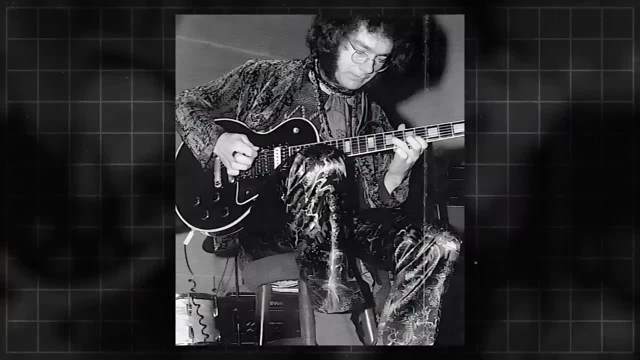 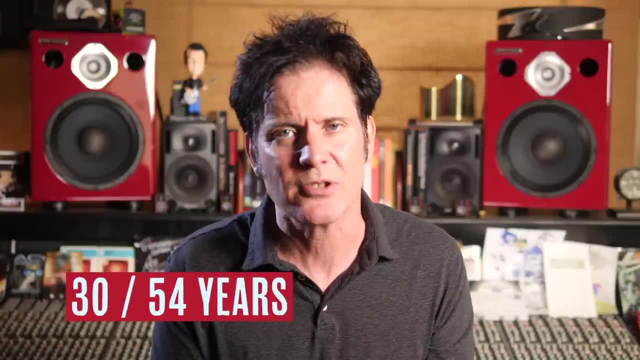 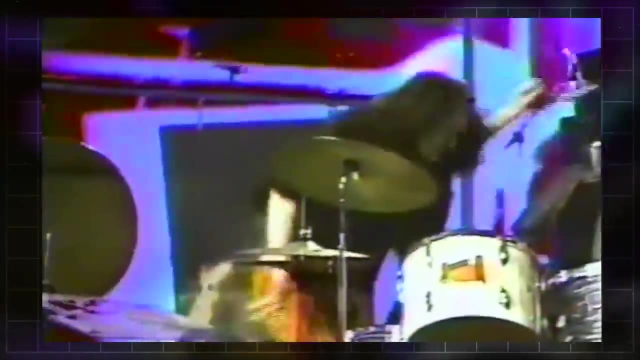 leader and only continuous member. The band has had four long hiatuses. The band has been active for about 30 out of those 54 years. New lineups to King Crimson often played into a musical style that is completely different from that of its previous incarnations. This was in part due to the continuously changing 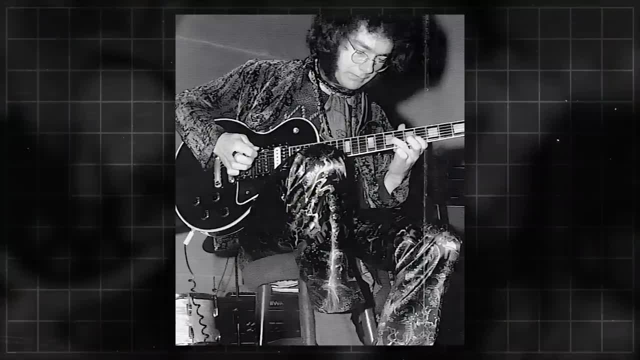 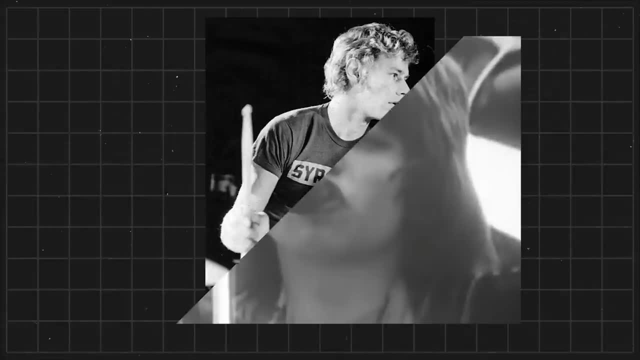 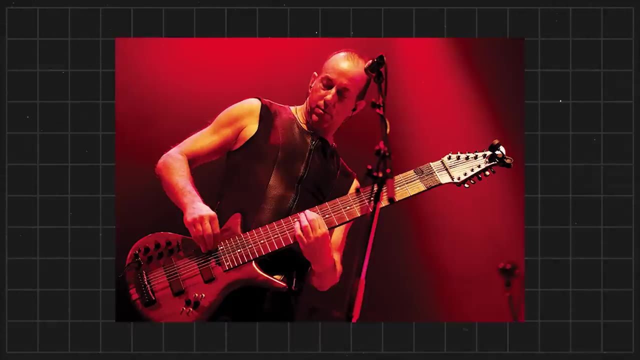 musical visions of Robert Fripp, but also because of the particular talents of the musicians involved. Over these years have included well-known players like Greg Lake, Bill Bruford, John Whetton, Adrian Ballew and Trey Gunn, and the current lineup includes top musicians like Tony Levin, Pat Mastolotto. 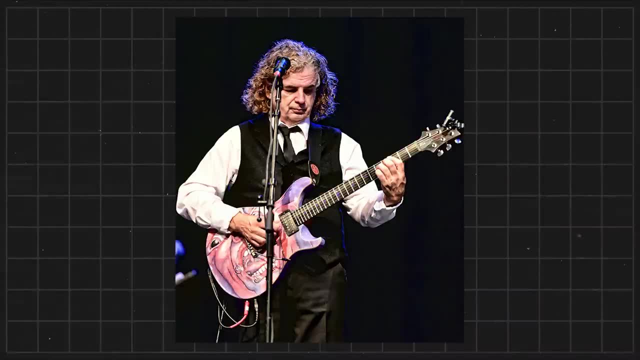 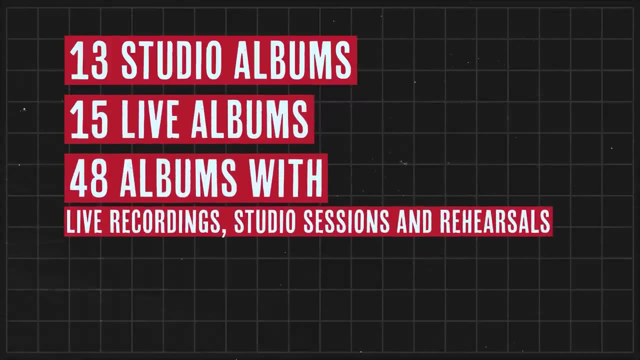 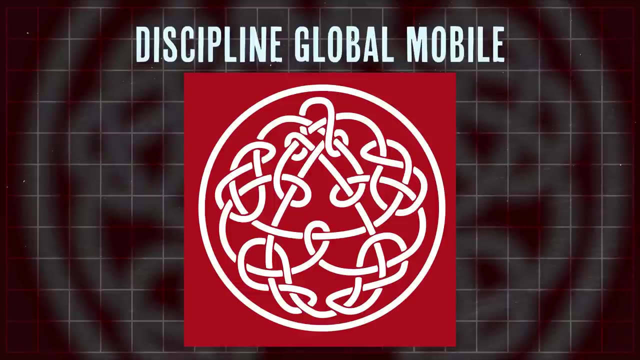 and Jacko Jackchick. Over the three decades of its existence, King Crimson has released 13 studio albums, 15 live albums and 48 albums with live recordings, studio sessions and rehearsals. Many of these albums are issued by Fripp's label, which he has called. 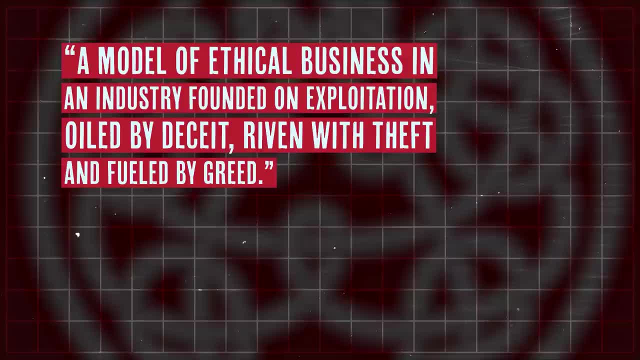 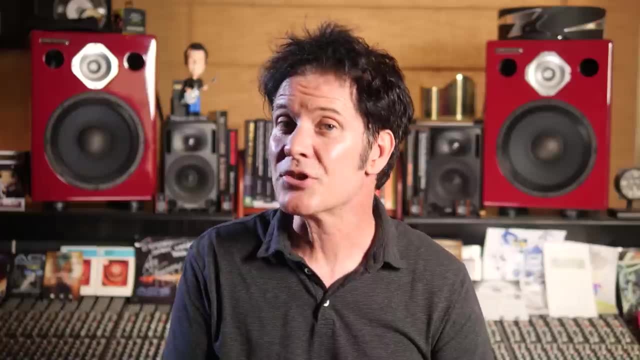 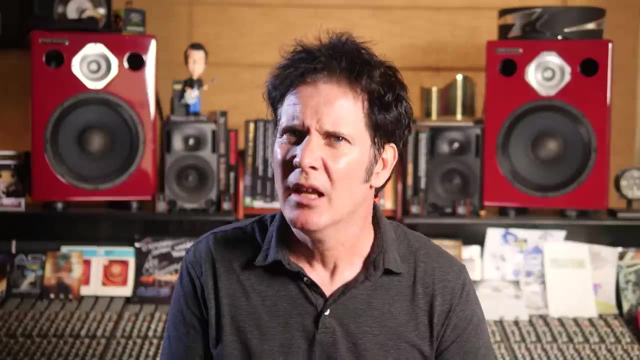 a model of ethical business in an industry founded on exploitation, oiled by deceit, riven with theft and fueled by greed. The legacy of King Crimson and of Fripp's innovative and very distinctive guitar playing is enormous. It was foundational to the prog rock genre, with all related British bands including Yes. 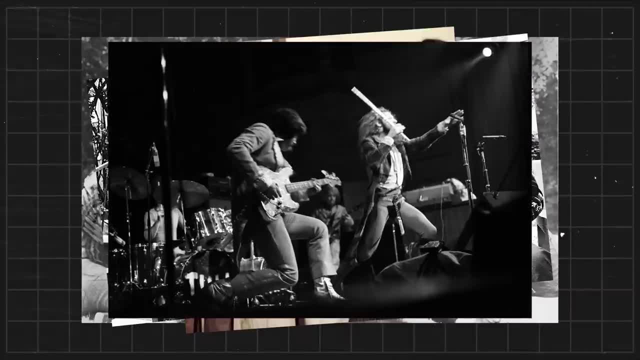 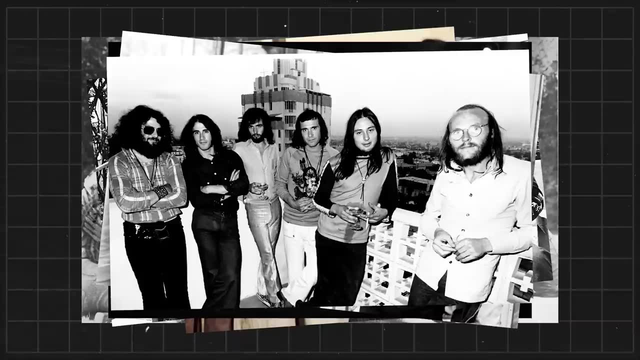 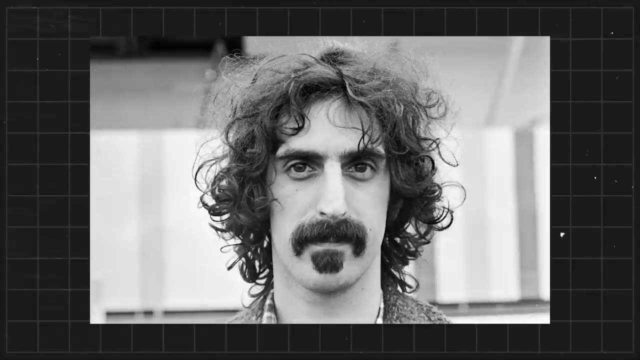 Genesis, Emerson Lake & Palmer, Jethro Tull, Van de Graaff, Generator, Gentle Giant and countless others owing a huge debt. King Crimson and Fripp also influenced grunge, post-punk, new wave and acts like Frank Zappa, David Bowie. 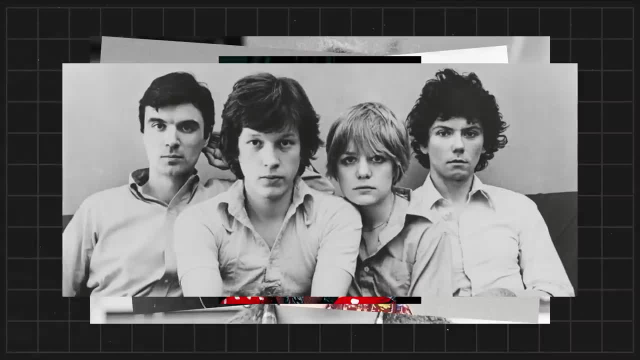 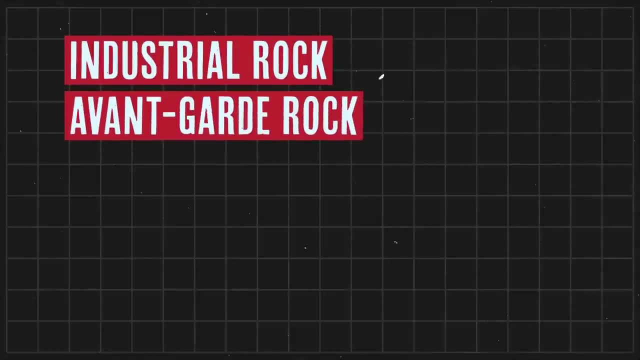 Peter Gabriel, Brian Eno, Talking Heads and many more. King Crimson continues to be regarded as one of the forefathers of today's industrial and avant-garde rock and of progressive metal and heavy metal, The many different incarnations of 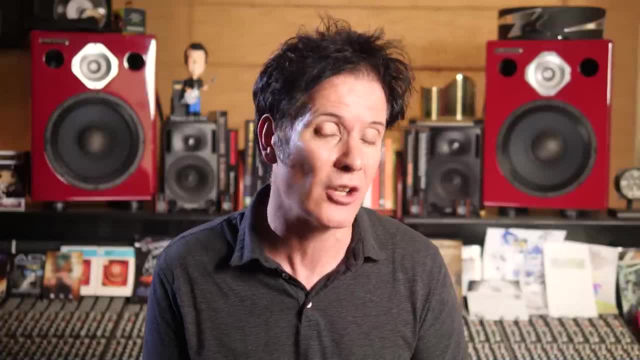 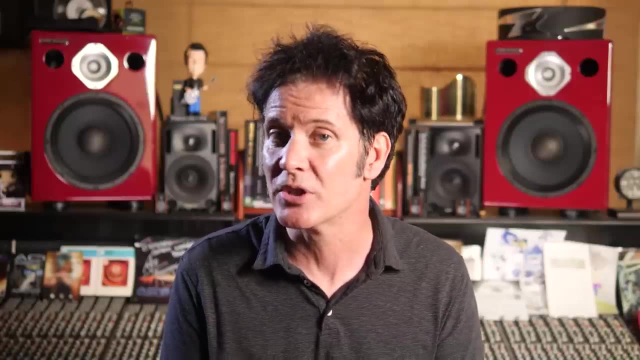 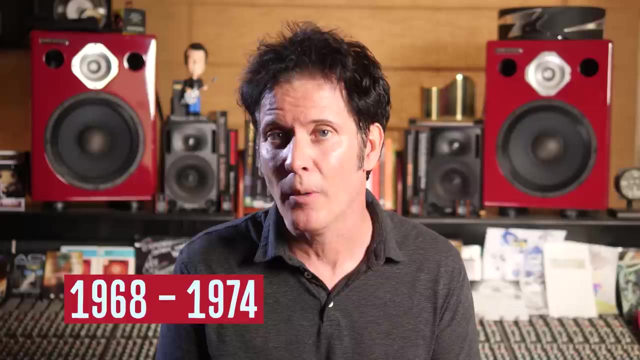 King Crimson and the radically different kinds of music each incarnation played resulted in an oeuvre of stunning diversity. It warrants breaking up our discussion of King Crimson into two videos. In this video we will look at the period 1968-1974.. 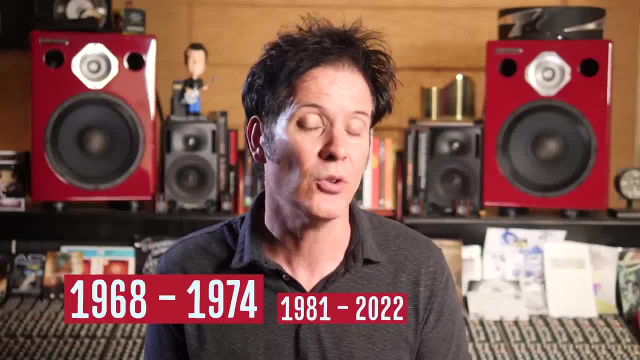 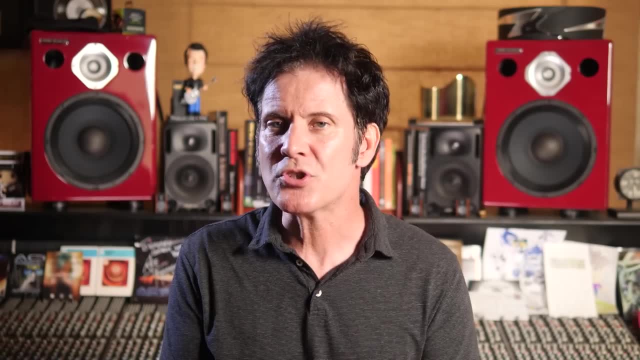 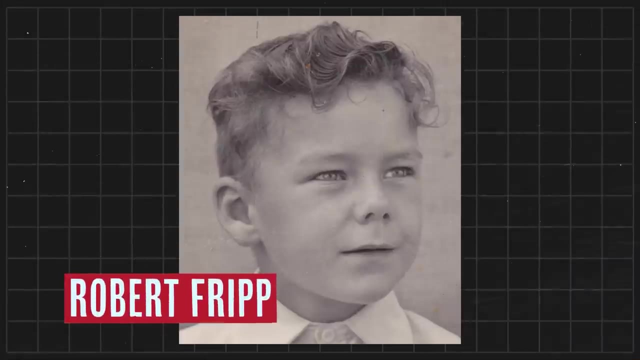 In part two we'll look at the band from 1981 until today. The origins of King Crimson can be traced back to Wimborne Minster, a small town in Dorset in southwest England, where Robert Fripp was born in 1915.. 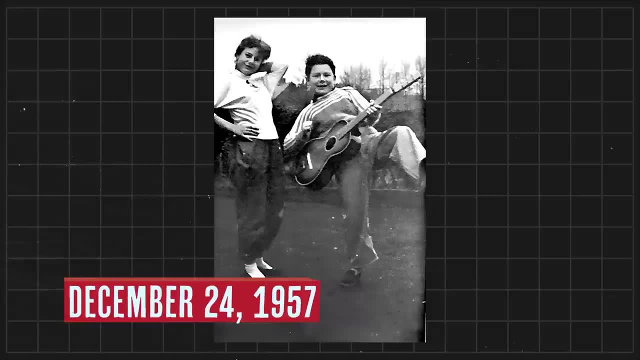 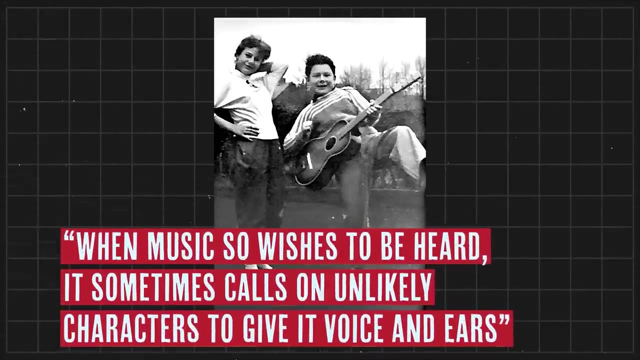 His parents gave him a guitar on December 24, 1957, when he was eleven. He has said that he immediately knew the instrument would be his future, despite also claiming that he started out tone-deaf, with no sense of rhythm. His later statement: when music so wishes to be heard, it sometimes calls on unlikely characters. 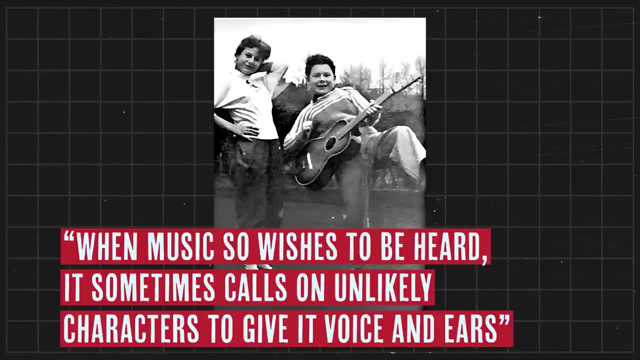 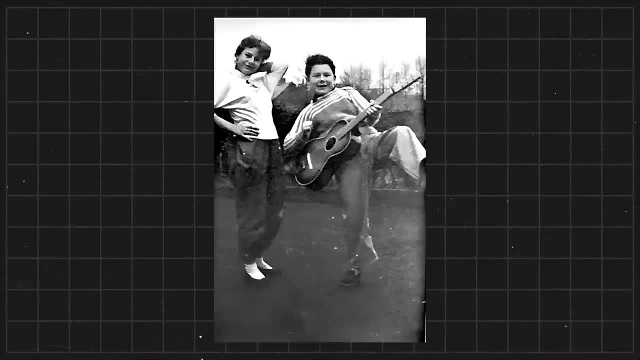 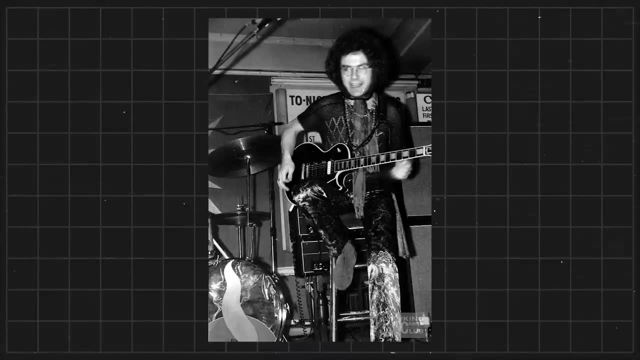 to give it voice and ears seems to apply first and foremost to himself. Fripp received guitar lessons from two local teachers, one of whom taught him cross-picking, which became an important feature of his later style. Fripp's early musical influences were unusually wide-ranging. 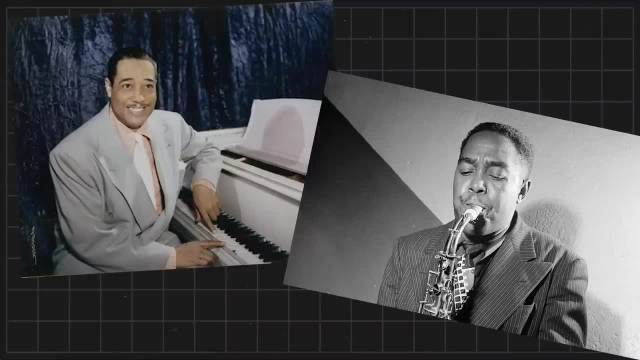 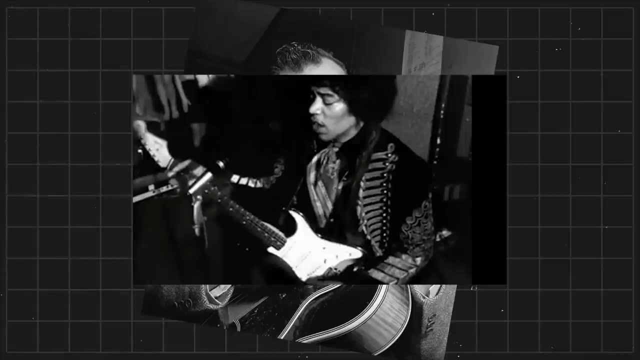 and included jazz musicians like Duke Ellington and Charlie Parker, Elvis guitar player Scotty Moore and, a little later, Django Reinhardt, Jimi Hendrix and classical composers like Antonin Dvořák, Béla Bartók and Igor Stravinsky. 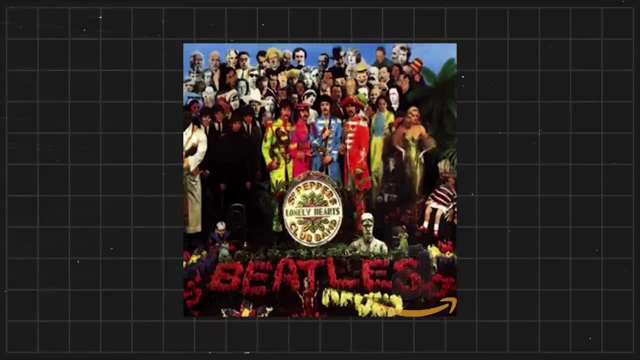 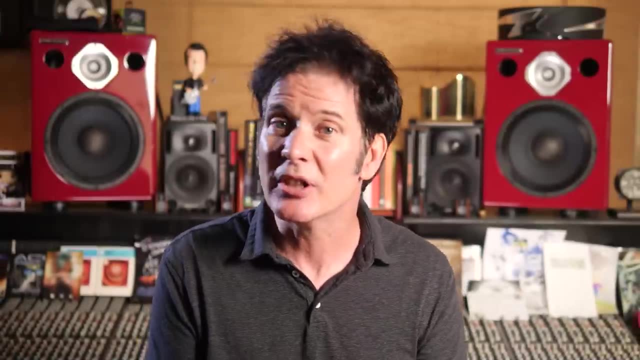 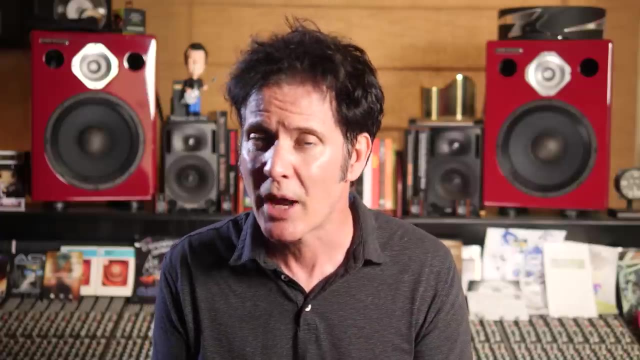 The music and production concepts of the Beatles' Sgt Pepper's Lonely Hearts Club band were also of particular interest to him. Fripp played in various bands during his formative years, including the Ravens and the jazz band Majestic Dance Orchestra. In 1967, he joined forces with two brothers, drummer Michael Giles and bassist Peter Giles. 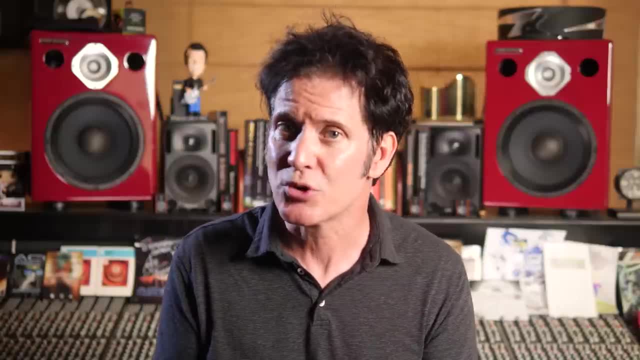 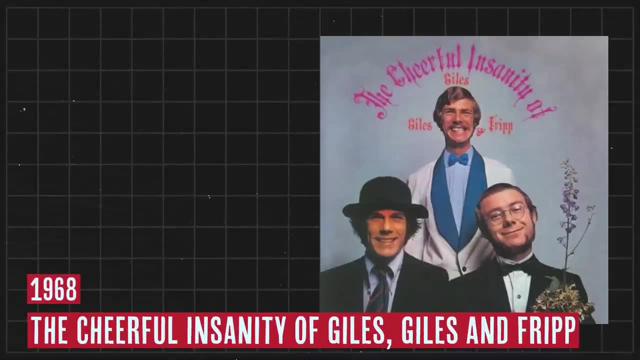 The trio moved to London and recorded one album at Deco Studio No 2, called The Cheerful Insanity of Giles, Giles & Fripp, which contained whimsical folk and psychedelic pop. When Giles, Giles & Fripp failed to find success, Peter Giles left. 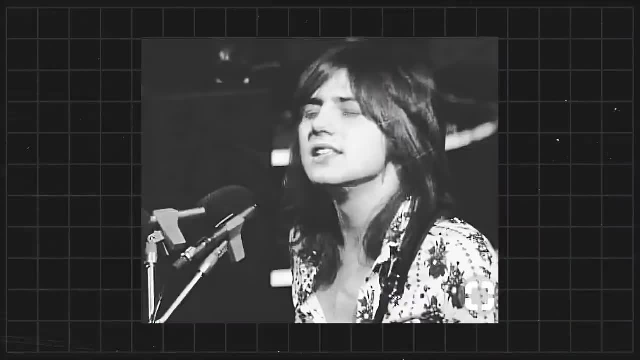 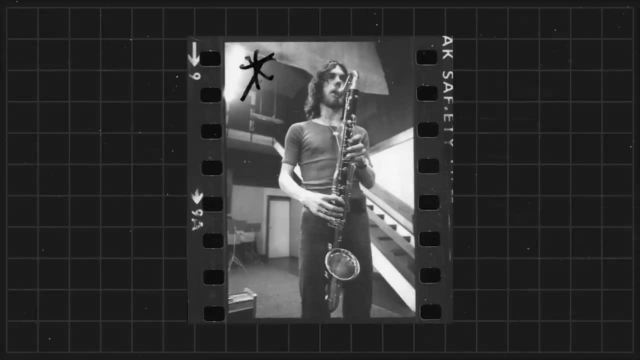 and was replaced by bassist and singer Greg Lake, a friend of Fripp from the Dorset days. Saxophone, flute and keyboard player Ian MacDonald also joined and he introduced the band to Peter Sinfield, a computer programmer and a poet. 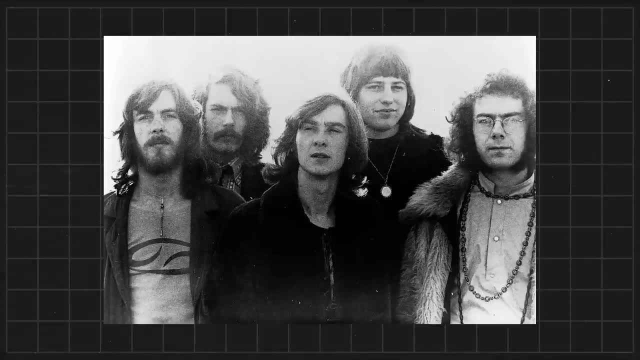 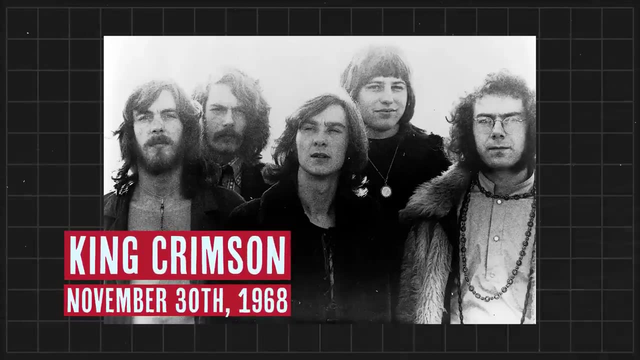 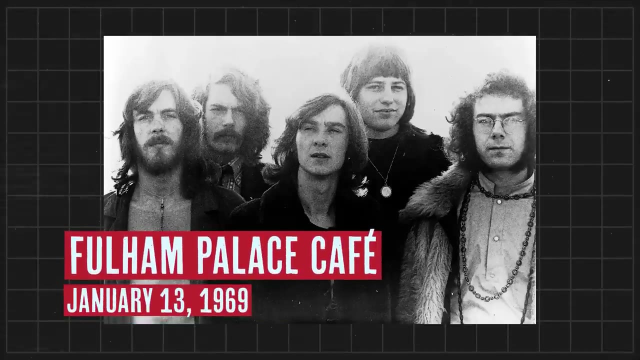 The quintet of Michael Giles, Greg Lake, Ian MacDonald, Peter Sinfield and Fripp decided to call itself King Crimson on November 30, 1968.. Their first rehearsal took place on January 13, 1969, in the basement of Fulham Palace Cafe in West London. 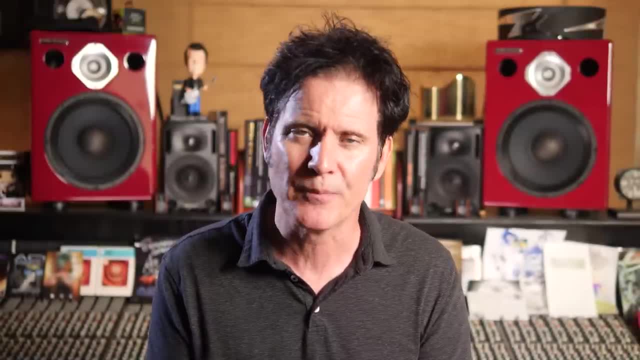 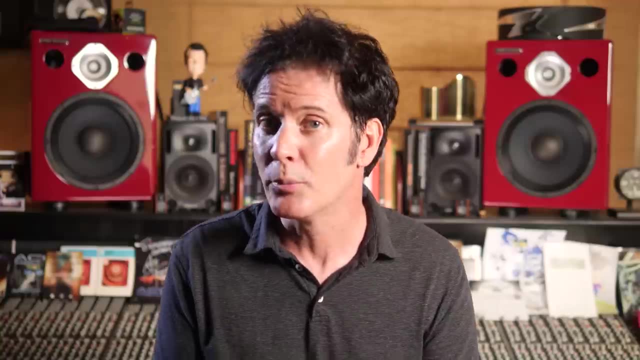 The quintet immediately took a radical new musical route. Both Fripp and MacDonald had a great interest in classical music and wanted to incorporate this into the band's music. The four musicians in the band were also very accomplished on their instruments and were keen to stretch out. 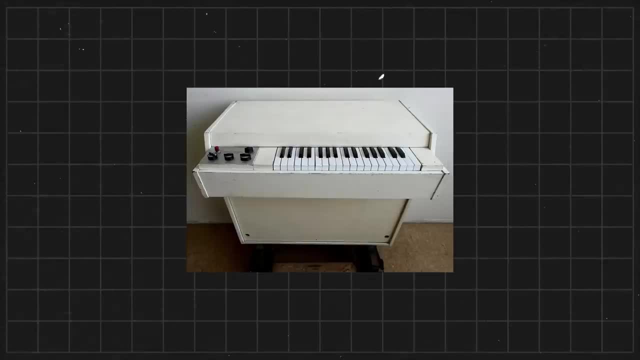 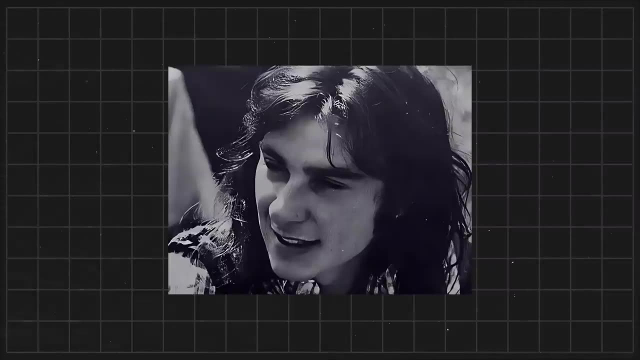 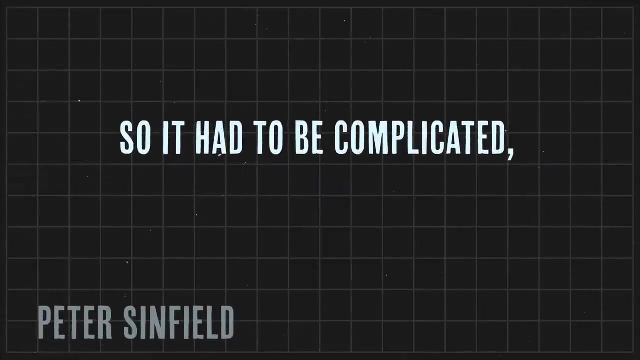 McDonald brought a Mellotron keyboard which became a crucial ingredient of the sound of the band. Sinfield was tasked with writing lyrics and album cover and stage-like design. He observed the band's rehearsals and noted If it sounded at all popular. it was out, So it had to be complicated. 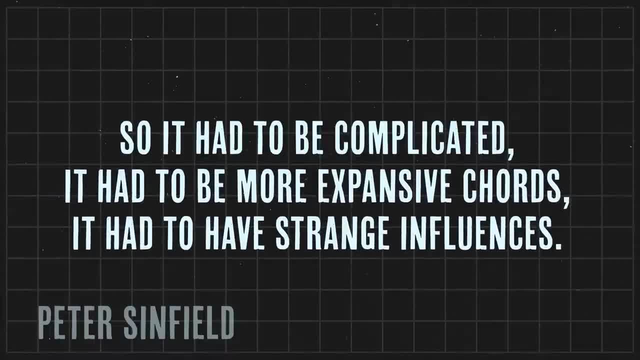 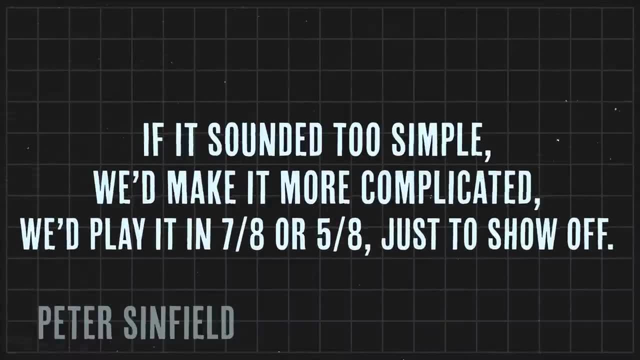 It had to be more expansive chords. It had to have strange influences. If it sounded too simple, we'd make it more complicated. We'd play it in 7-8 or 5-8, just to show off. The band spent three months working hard at writing and practicing new material. and made its debut at London's Speakeasy Club on April 9, 1969.. The magic of the band and the material they had written was immediately apparent and they very quickly became undeniable. On July 5,, the band performed at a free concert in Hyde Park in central London. 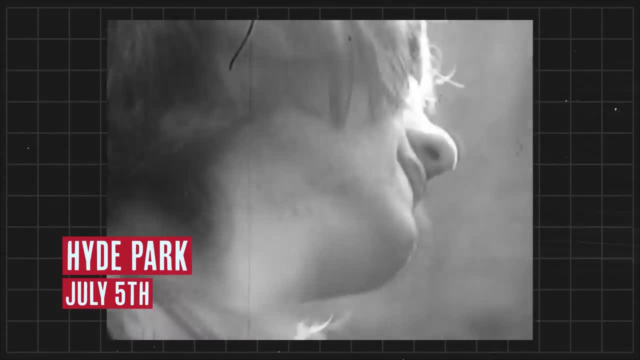 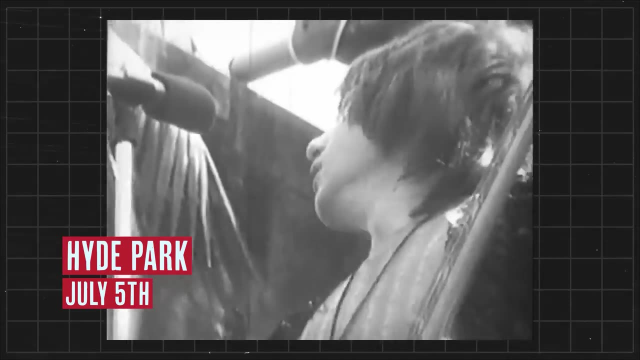 a support act to the Rolling Stones. By the time King Crimson had ripped through an incendiary and high-speed version of their song 21st Century Schizoid Man, half a million mouths were agape and everyone in the audience knew a spectacular new act had arrived. 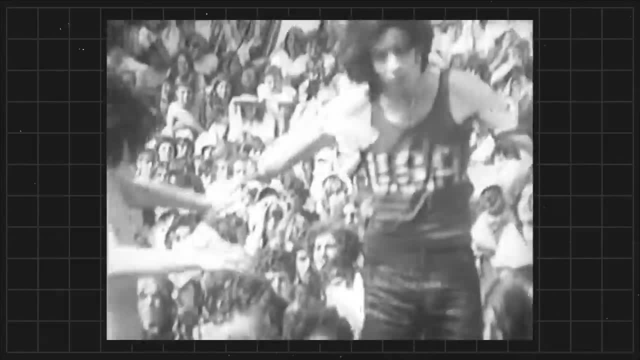 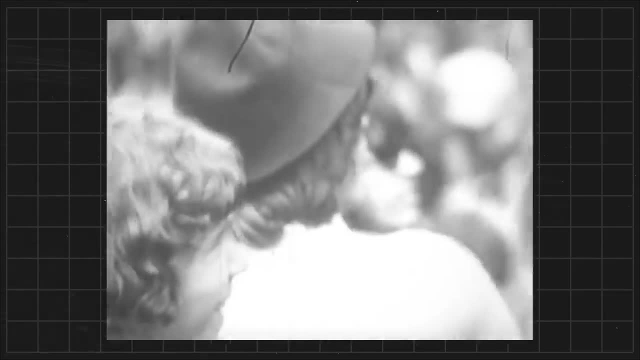 It's hard to overstate the importance of the iconic Hyde Park gig And when they walked off the stage, the band was aware that something amazing had just happened. Fripp noted in his diary that day Mammoth success of importance which will take time to appreciate. 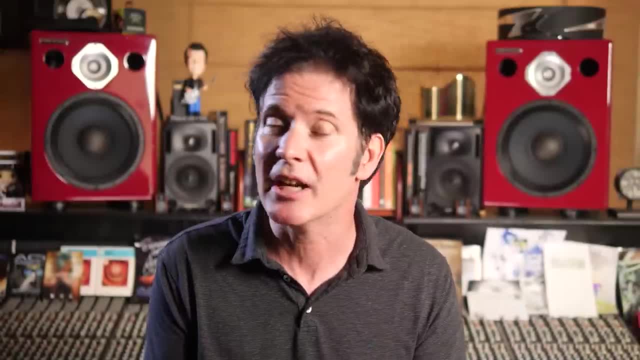 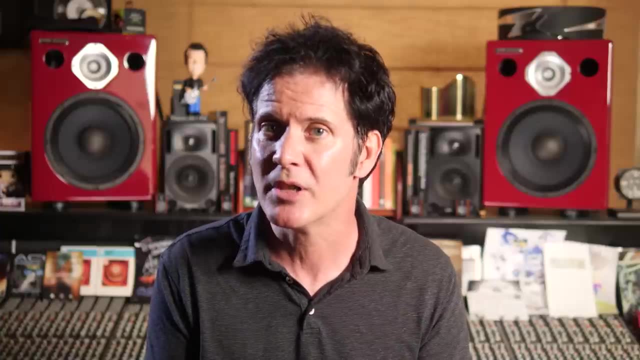 The recognition did not stop here. The band performed four days later at the Revolution Club in Mayfair in North London With Jimi Hendrix present. He walked up to Fripp afterwards and complimented him on the performance. Fripp later learned from someone who sat next to Hendrix that the American 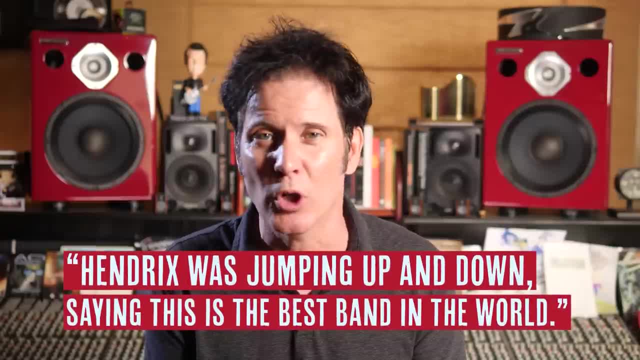 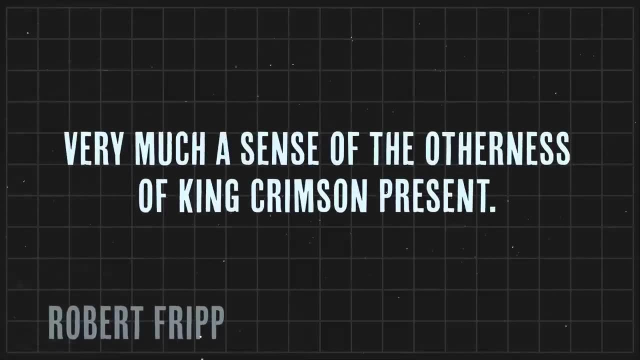 had been jumping up and down saying this is the best band in the world. Many years later, Fripp recalled that in 1969, the band members had very much a sense of otherness, of King Crimson present. It was referred to as a good fairy or the moving spirit. 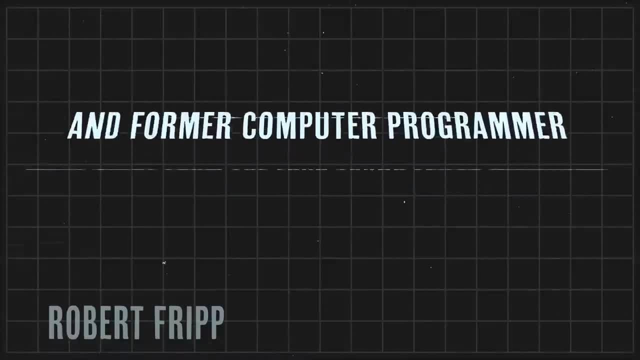 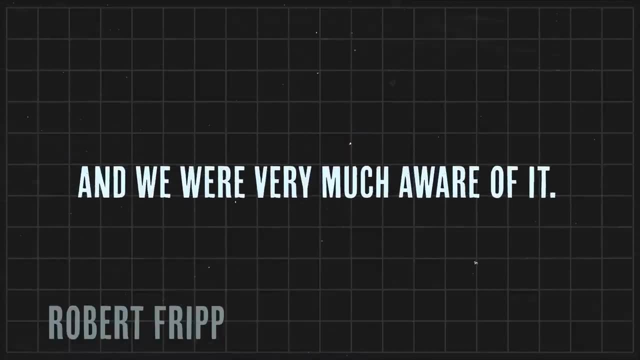 There was something quite apart from the four young failed musicians and former computer programmer Peter Sinfield, who wrote words and played very bad guitar, And we were very much aware of it By this point. King Crimson had signed a management and a record deal with EG Management. 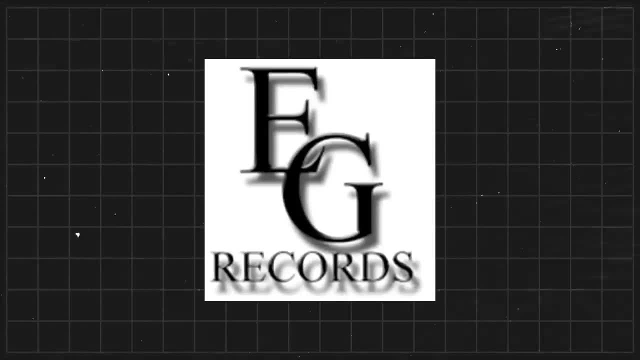 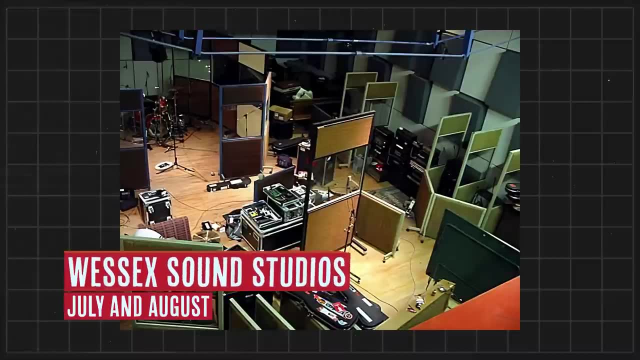 and was working on its debut album. There were sessions with Moody Blues producer Tony Clark, which did not work out. Eventually, the band's debut album was recorded during July and August at Wessex Sound Studios in North London to one-inch eight-track with Robin Thompson Engineering. 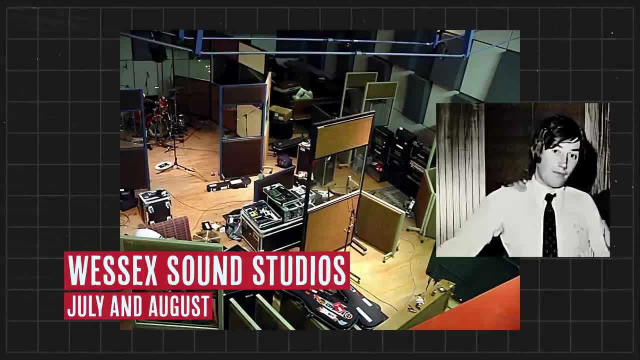 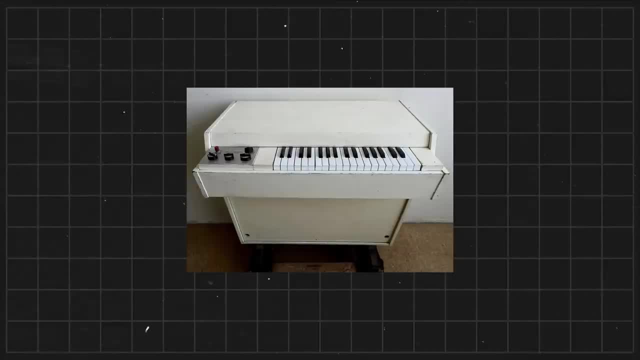 Unusually for the time, King Crimson produced the recording themselves. They were aware that the sound of the Mellotron was crucial and Ian Macdonald repeatedly overdubbed the keyboard instrument and also his saxophone and flute, sometimes using five generations of tape to achieve the depth of sound they were after. 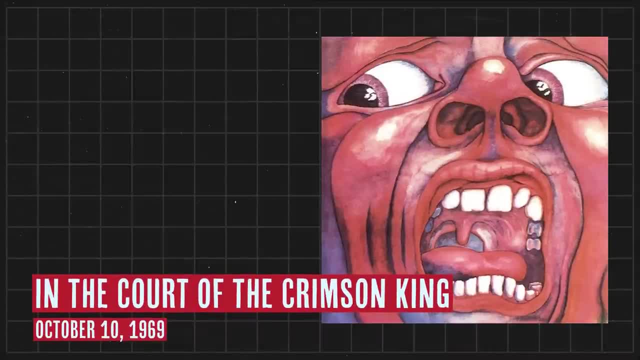 In the Court of the Crimson King was released on October 10, 1969,, and while The Who's, Pete Townshend, immediately called it an uncanny masterpiece, critics were initially guarded, However, helped by the startling cover painted by computer programmer Barry Godber. 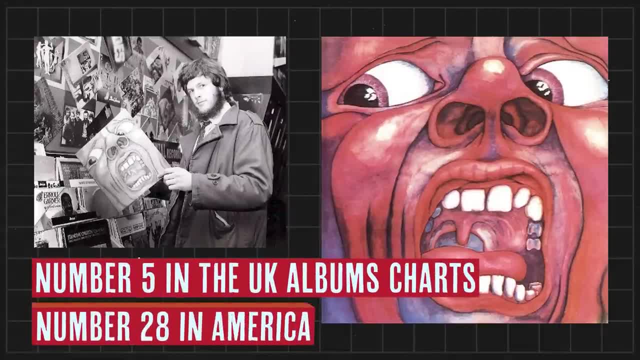 it climbed to number five in the UK albums charts and number 28 in America Over the years. In the Court of the Crimson King has become universally recognised as a masterpiece. One critic has written that it blew the doors off musical convention and cemented those quintessentially British innovators'. 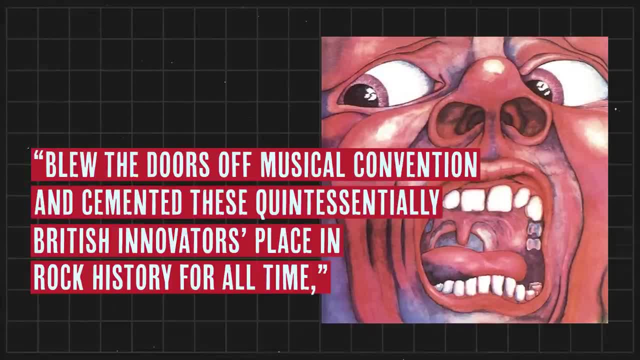 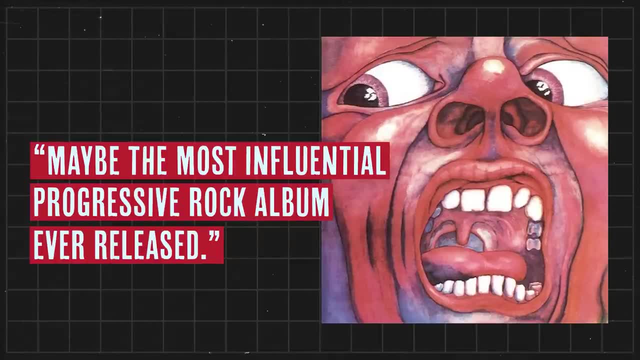 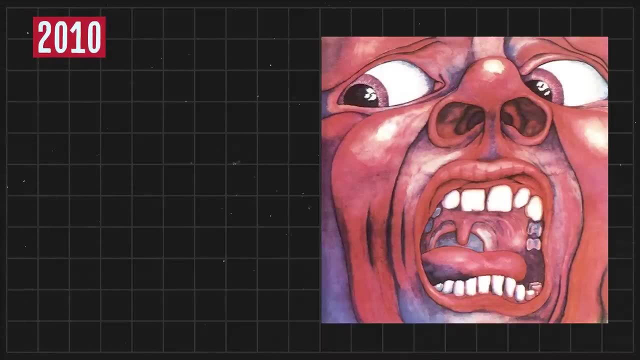 place in rock history for all time And another called it maybe the most influential progressive rock album ever released. The album came in second in a recent Rolling Stone list of greatest progressive rock albums of all time, and in 2010,, Kanye West sampled 21st Century Schizoid Man for his hit Power. 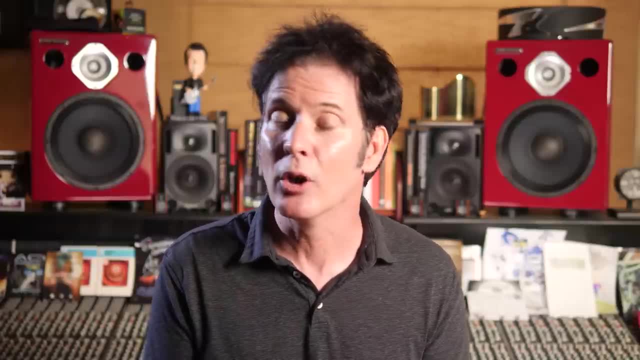 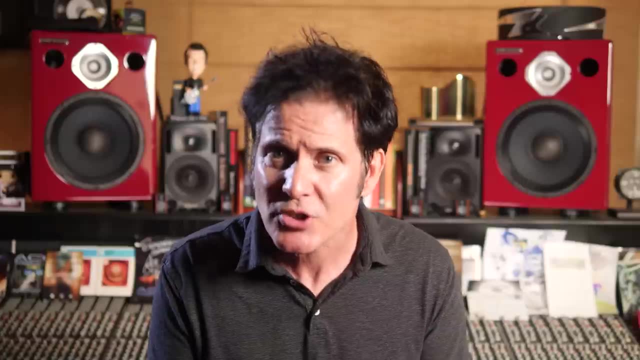 In the Court of the Crimson King is, in some respects, a tale of two albums. 21st Century Schizoid Man is a piece of spectacular proto-heavy metal that contains many of the characteristics that would be at the heart of much of King Crimson's later music. 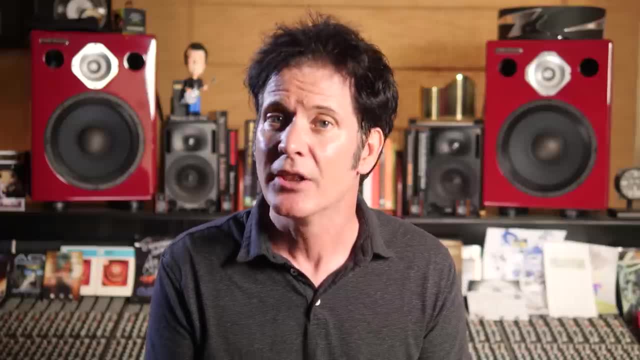 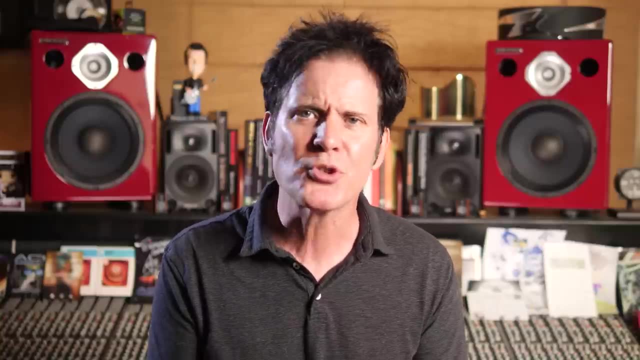 Most of all, there's a sheer visceral power of the track. There are also the industrial soundscape at the beginning, the abrupt switches in dynamics, tempo and mood, the multitude of instrumental colours, Fripp's screeching guitar solo in the middle. 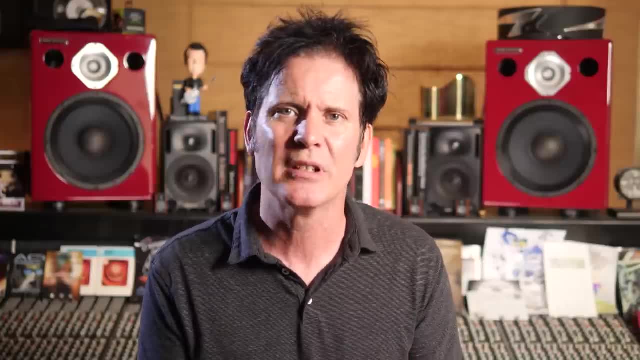 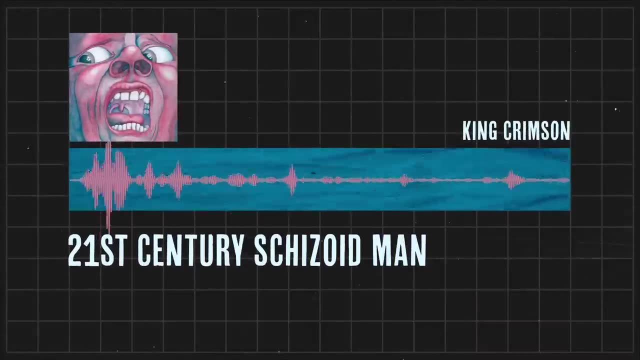 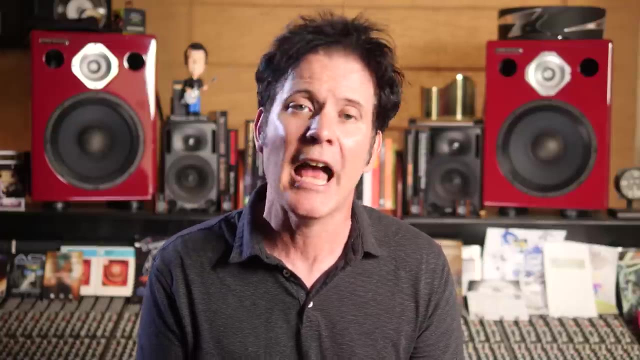 with sustained notes and unusual and often large intervals and the free jazz chaos at the end. Other pieces on the album used the Mellotron extensively and incorporated gentle folk, symphonic rock and free jazz. King Crimson set the world of music alight in 1969. 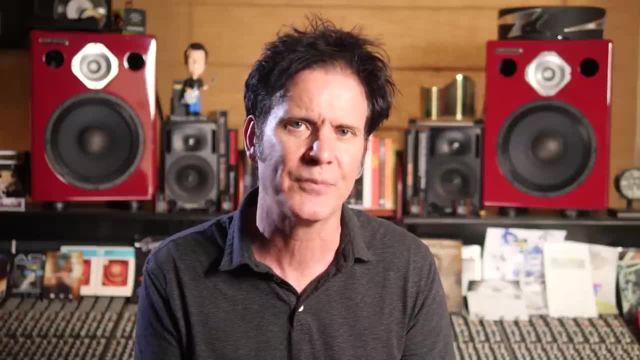 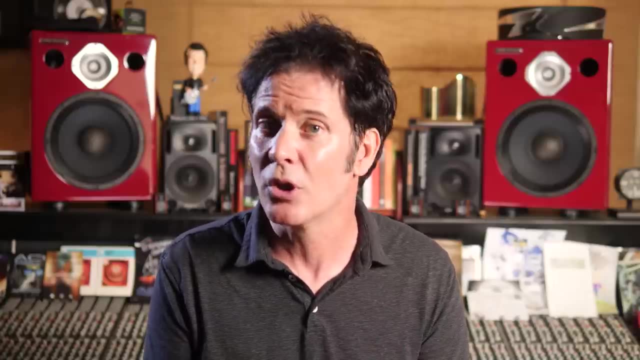 It was a stunning achievement that would prove to be difficult to sustain. It became increasingly apparent that Fripp was the driving creative force in the band and tensions and cracks started to show. MacDonald and Giles left the band at the end of 1969 after their first US tour. 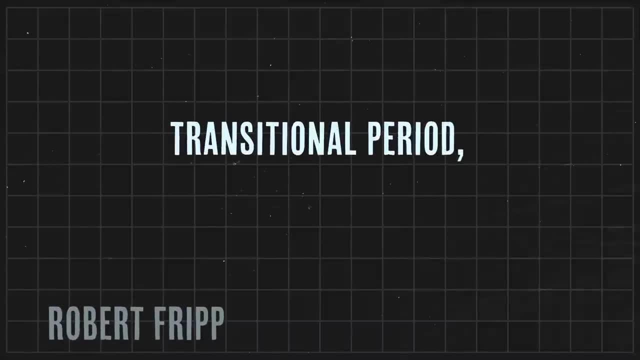 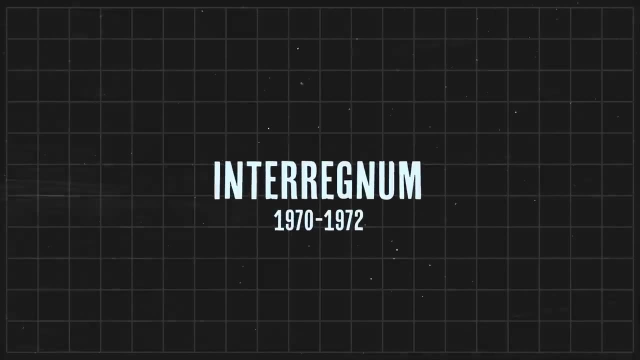 Fripp later explained that the band had entered a transitional period during which it was important for King Crimson to remain alive. The period has been called interregnum and lasted from the beginning of 1969, until the middle of 1972. 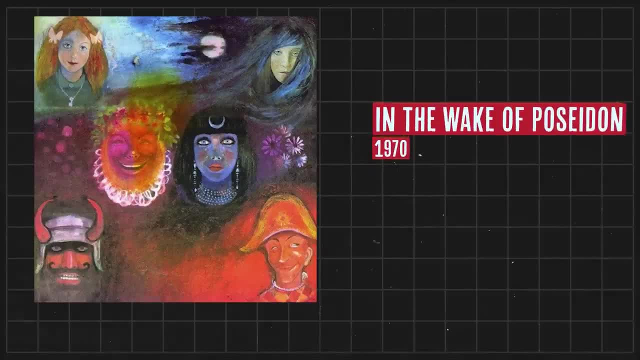 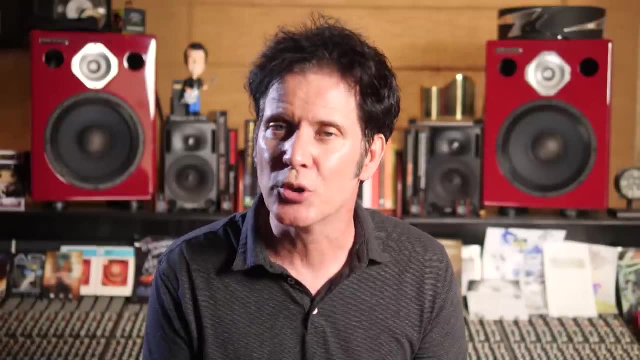 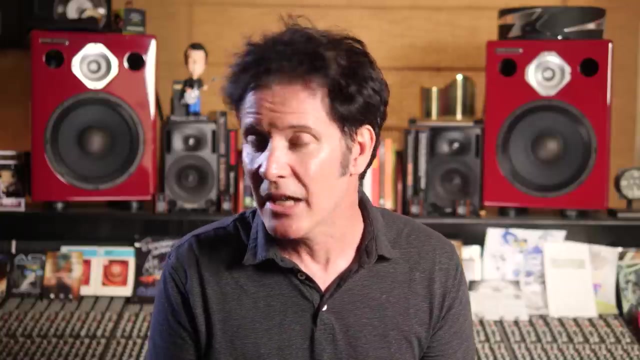 During these years, three albums were recorded In the Wake of Poseidon, Lizard and Islands. Fripp and Sinfield were the two main members, with the guitarist writing all the music, and the latter, the words In the Wake of Poseidon, was again recorded at Wessex Studios. 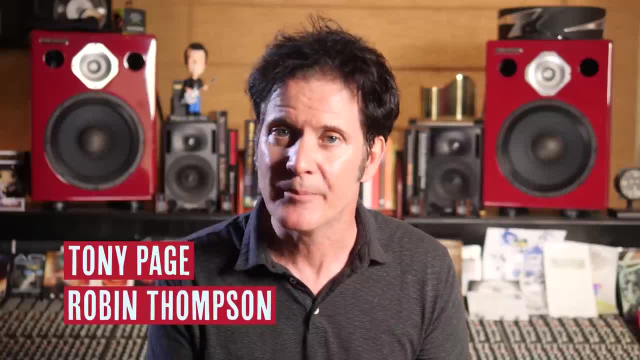 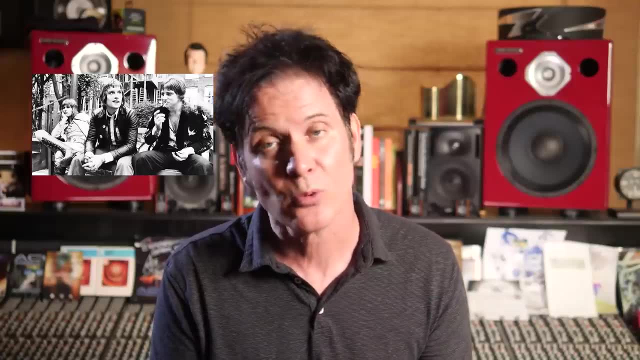 with Tony Page and Robin Thompson engineering Greg Lake by this stage agreed to join Emerson Lake and Palmer, But after Fripp turned to music, Fripp turned down two unknown singers, one called Elton John and the other Brian Ferry. 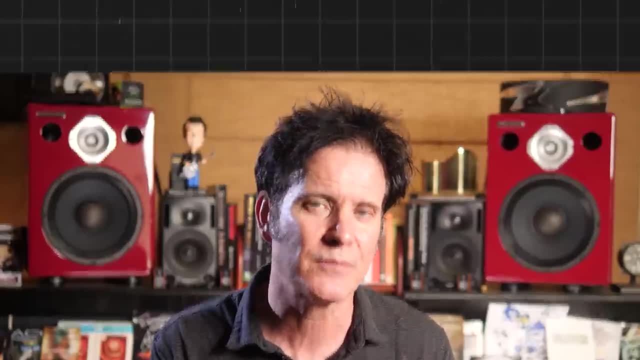 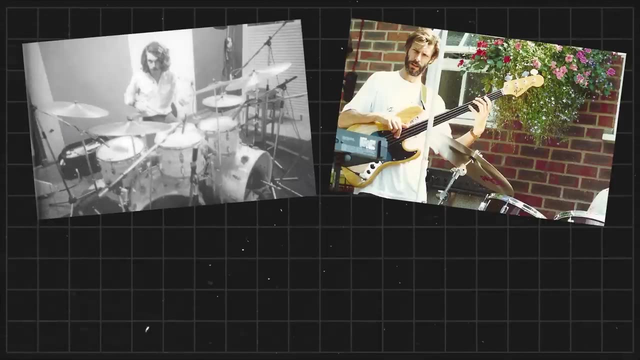 Lake agreed to sing most of the songs as a special guest. Michael and Peter Giles were also enlisted as guest musicians on drums and bass and were joined by avant-garde pianist Keith Tippett and saxophonist and flautist Mel Collins. 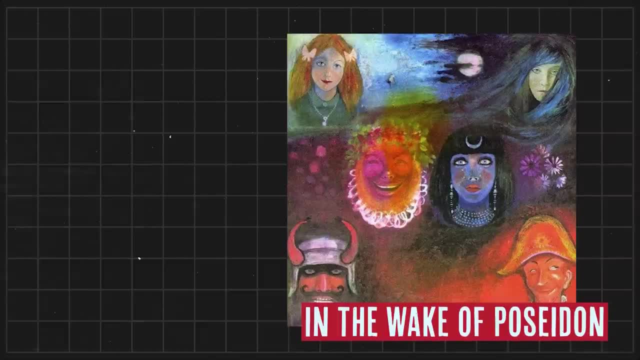 The music on In the Wake of Poseidon lacks the visceral power of 21st century schizoid man and contains music with predominantly classical folk and jazz rock elements. Standout tracks are Pictures of a City, Cat's Food and The Devil's Triangle. 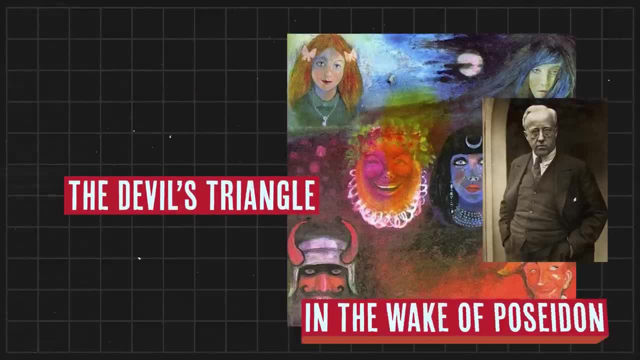 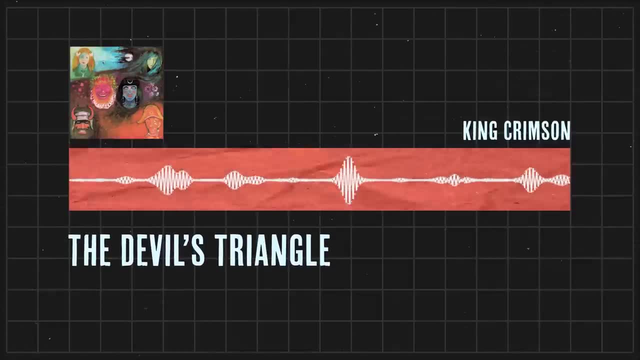 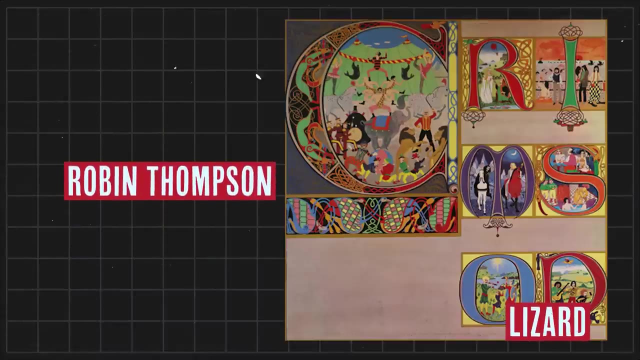 The latter is in part a reworking of Gustav Holst's Mars Bringer of War of the famous orchestral work The Planets. The next album, Lizard, was also recorded at Wessex Sound with Robin Thompson, again engineering. 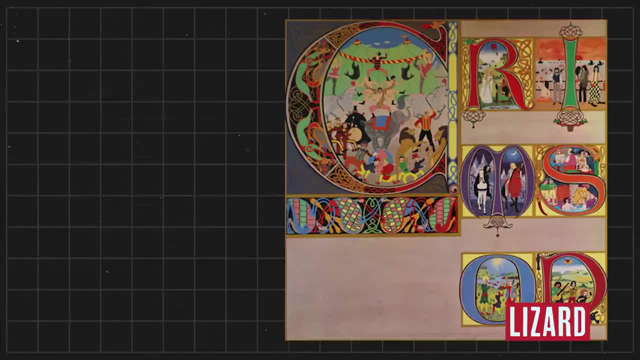 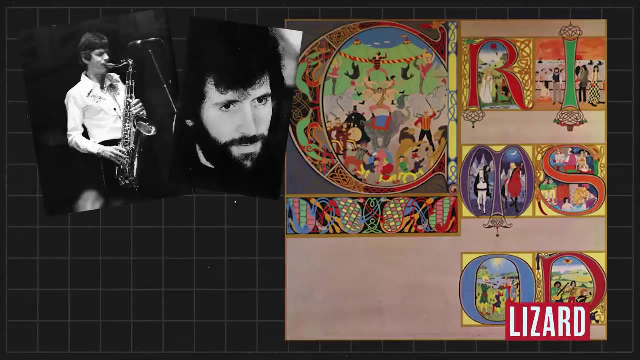 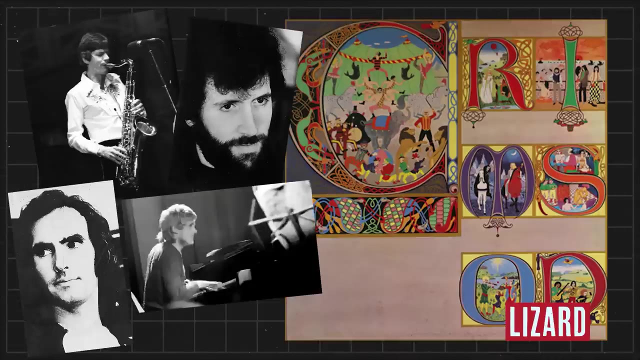 And the music is very much a development of the previous album. This time, King Crimson were extended to a complete band with Mel Collins on saxophone and flute, Gordon Haskell on bass and vocals and Andy McCulloch on drums. Keith Tippett appears again, plus there are three wind instrument players. 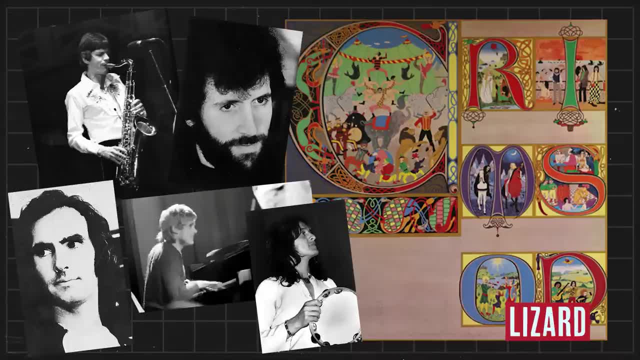 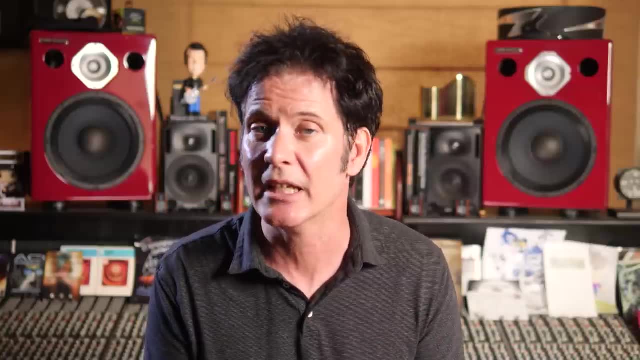 and John Anderson of Yes sings one track. Fripp himself has called the album unlistenable, but he later softened his opinion Unusually. the three King Crimson albums recorded during the Interregnum have become more appreciated over time and are now treasured as early precursors. 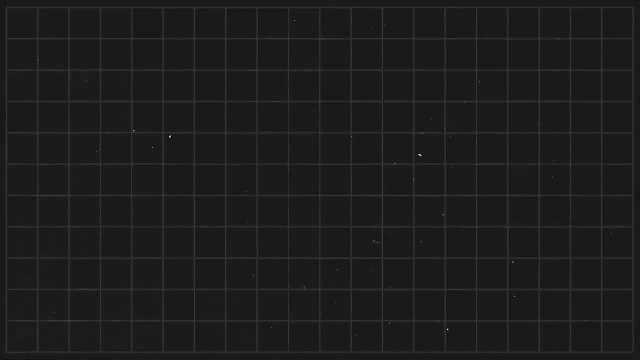 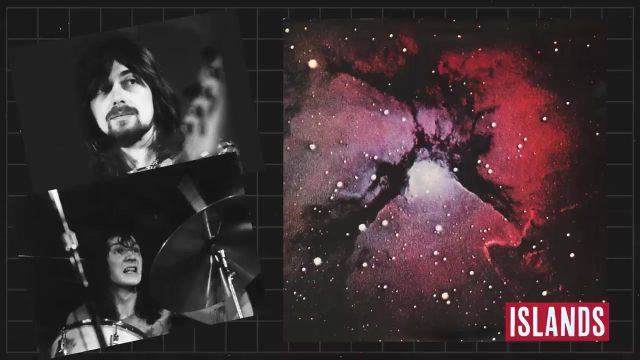 This is also the case with the third album, Islands, which featured a new rhythm section of bassist and singer Boz Burrell and drummer Ian Wallace, with again Keith Tippett on piano, as well as several orchestral musicians. 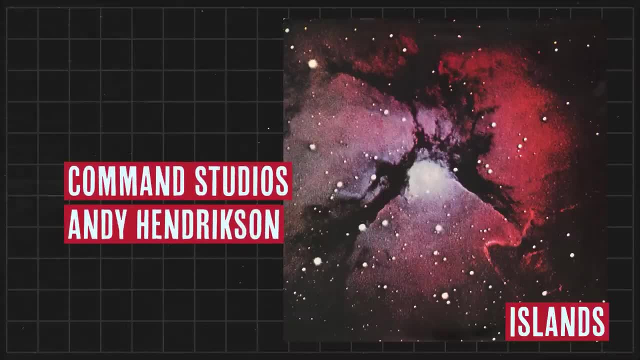 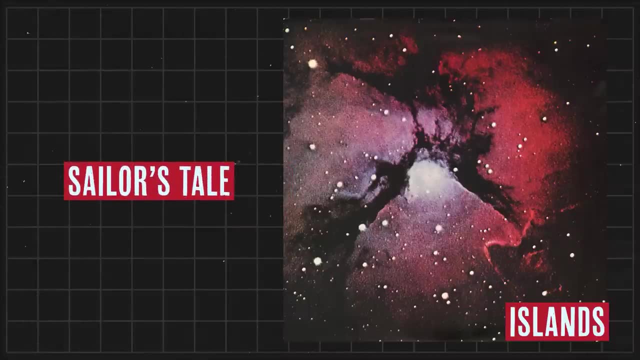 It was recorded at Command Studios by Andy Hendrickson. The music on Islands again has strong jazz, classical and folk influences. Sailor's Tale is a standout track featuring a circular bassline and Fripp's sustained electric guitar, Including an amazing guitar solo. 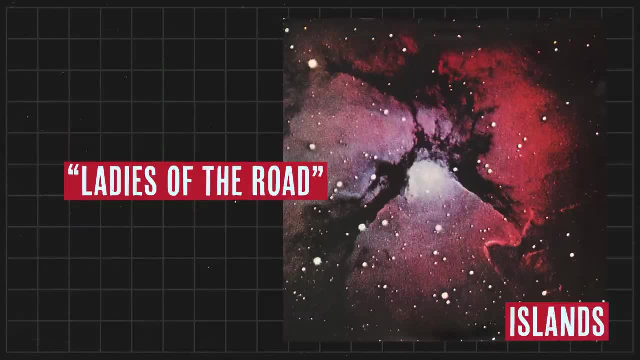 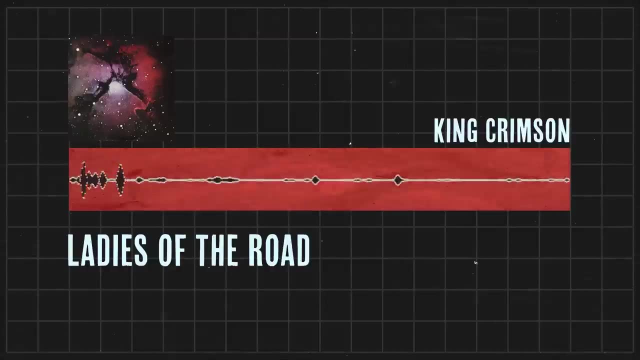 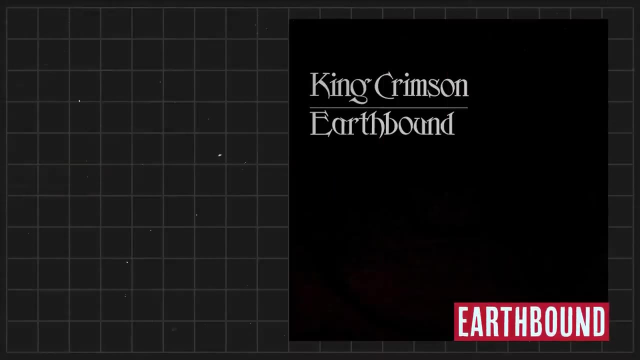 Ladies of the Road sounds like it's directly inspired by late era Beatles. In June 1972, King Crimson's first live album was released Earthbound, featuring the same band as On Islands. It had been recorded during the band's US tour. 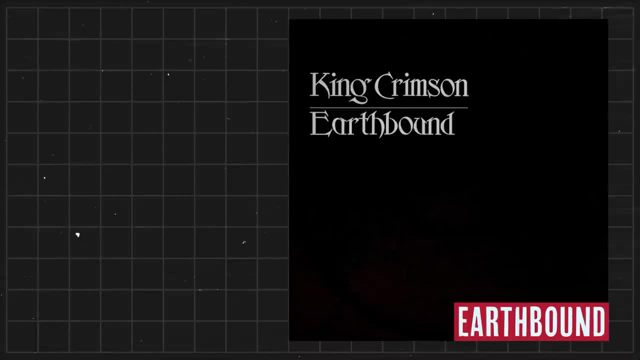 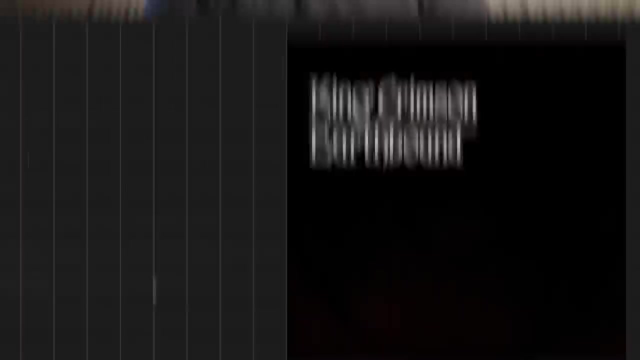 the beginning of 1972, on a stereo cassette recorder fed from a Kelsey Morris custom-built mixer, in the rain from the back of a Volkswagen truck. The album's poor sound quality has been widely criticized, but the intensity and ferocity of the performances were an indication of things to come. 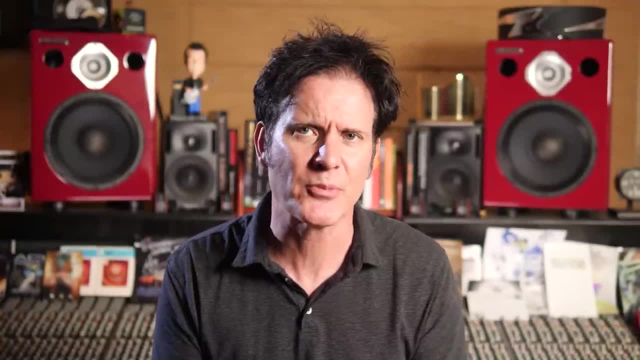 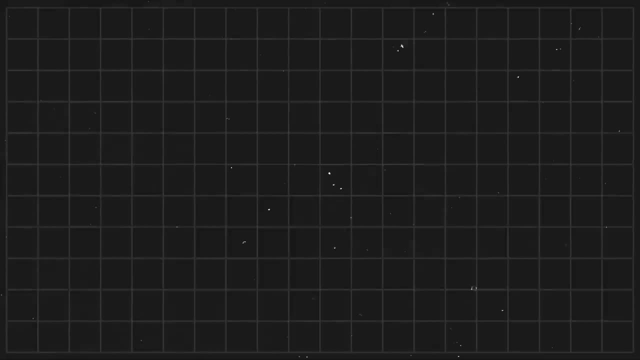 Robert Fripp was dissatisfied with the second incarnation of King Crimson and wanted to move the band into a more aggressive, avant-garde and rock-oriented direction. First on his shortlist was avant-garde percussionist Jamie Muir, who had worked with jazz rock guitarist Alan 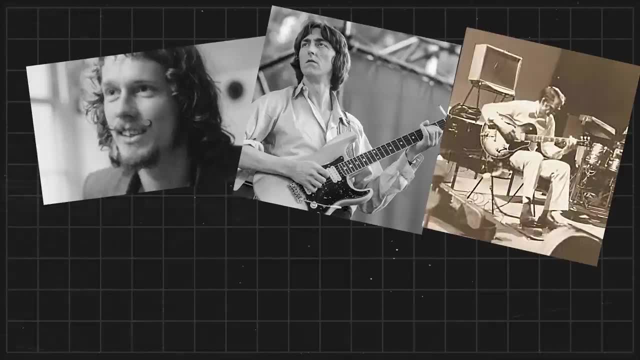 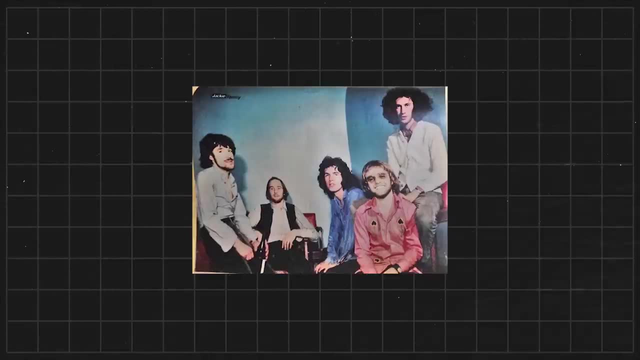 Holdsworth and avant-garde guitarist Derek Bailey. Next up was John Whetton, who Fripp knew from their Dorset days and who had worked in Family. Fripp also managed to convince Yes drummer Bill Bruford to abandon the successful prog rock band and switch to King Crimson. 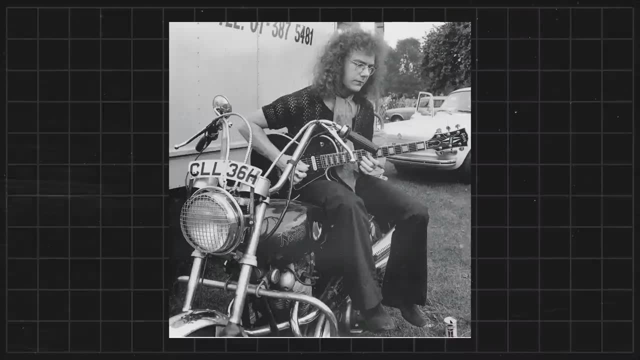 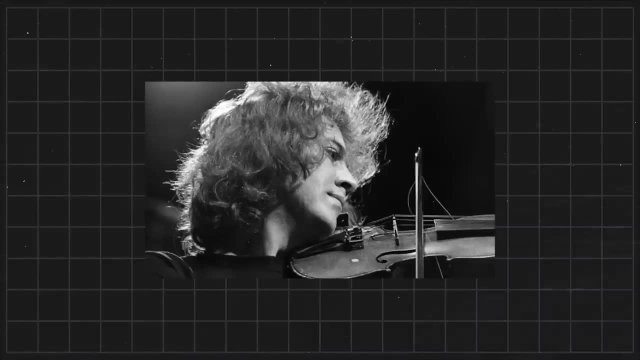 To eliminate the jazz leanings of the band, Fripp decided to go without a horn player and instead recruited classically trained violinist and keyboardist David Cross. The new quintet started rehearsals on September 4, 1972.. The same month, 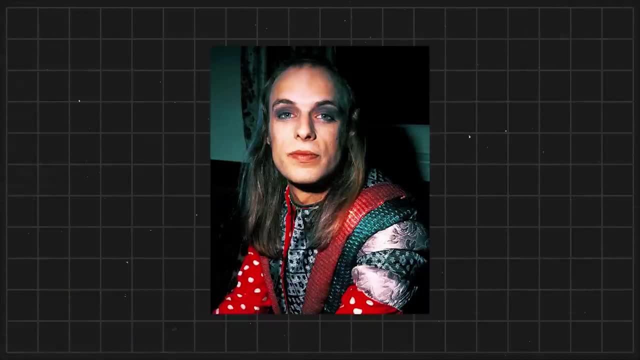 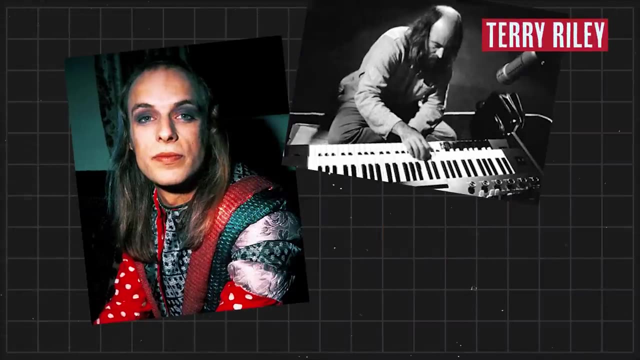 Fripp also worked for the first time with Brian Eno, who was still a member of Roxy Music. Eno was experimenting with a music creation system devised by composers Terry Riley and Pauline Oliveros that used two tape recorders to generate a long and gradually shifting tape. delay Using. 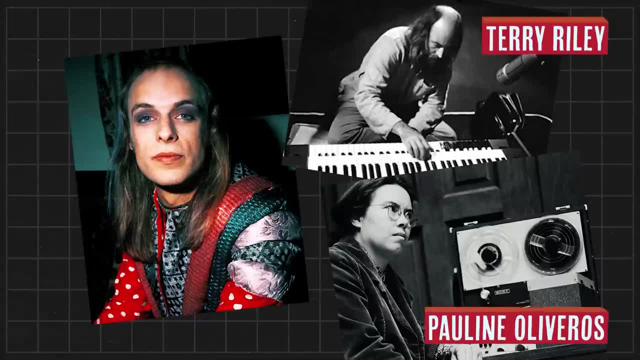 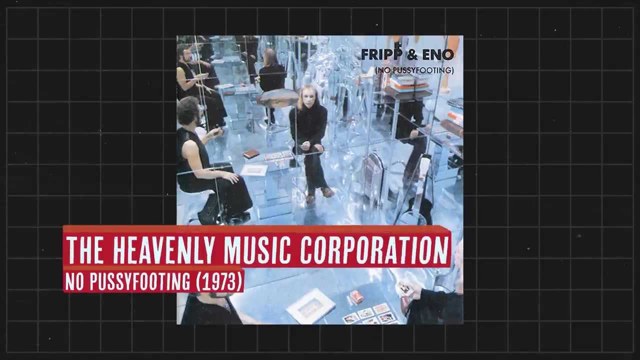 the system, Eno and Fripp came up with the ambient piece called the Heavenly Music Corporation. It appeared in 1973 on their duo debut album No Pussyfooting. The third incarnation of King Crimson played its first gigs in October of 1972. 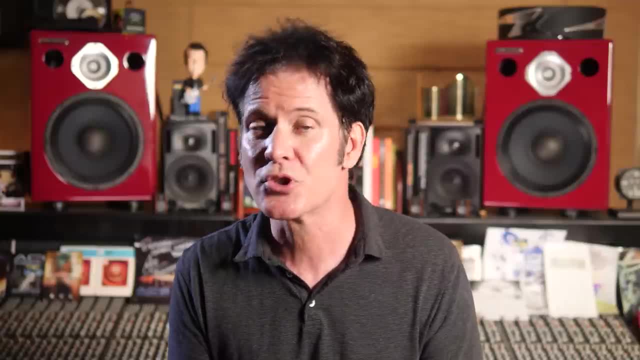 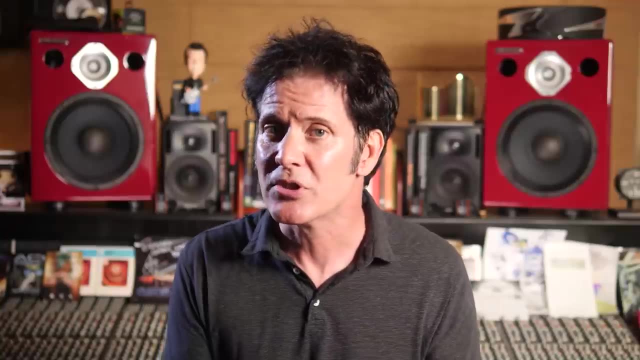 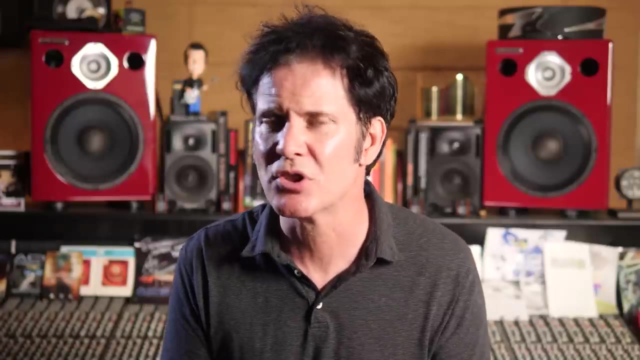 The band was writing and developing new material, often through on-stage collective improvisations, which tended to be atonal and without individual solos. More composed pieces featured lyrics written by Richard Palmer James, one of the founders of Supertrap. Fripp was extremely happy with the music of his new line-up. 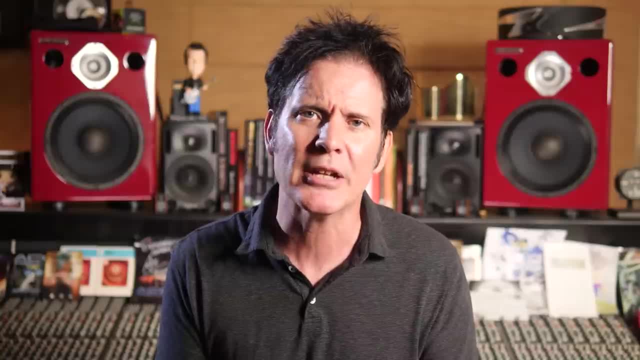 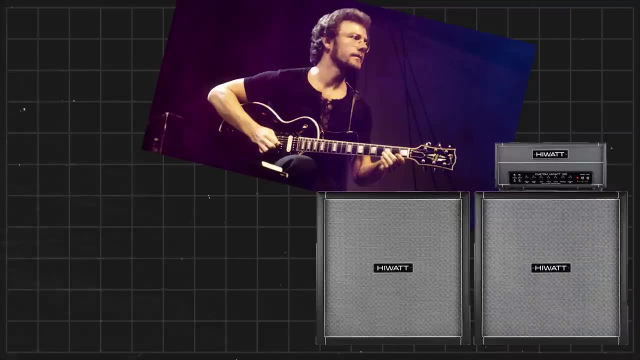 and widely declared that the magic of King Crimson had reappeared. At this point, Fripp performed on a Gibson Les Paul custom guitar with a hi-watt 100-watt amp and two 4x12 hi-watt speaker cabinets. He used fuzz volume and wah-wah pedals. 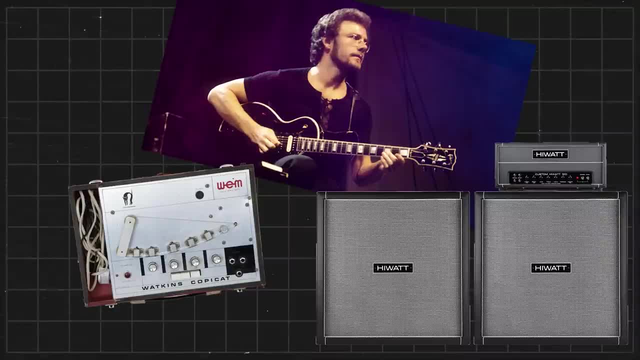 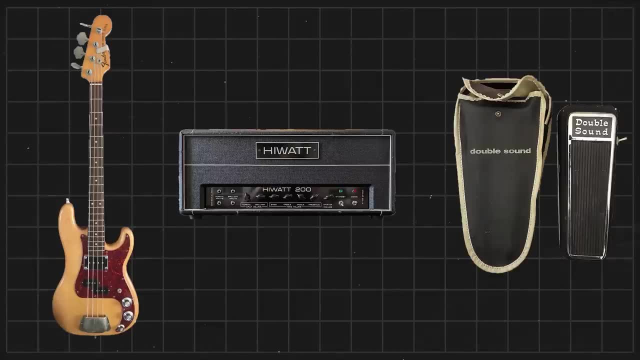 plus a Wham copycat echo unit. He also played a Mellotron 400.. John Whetton used a Fender Precision Bass with hi-watt amps and speakers, a double sound, wah-wah and fuzz pedal. David Cross played a violin. 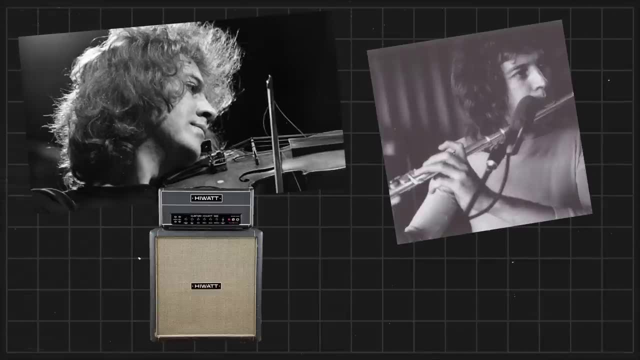 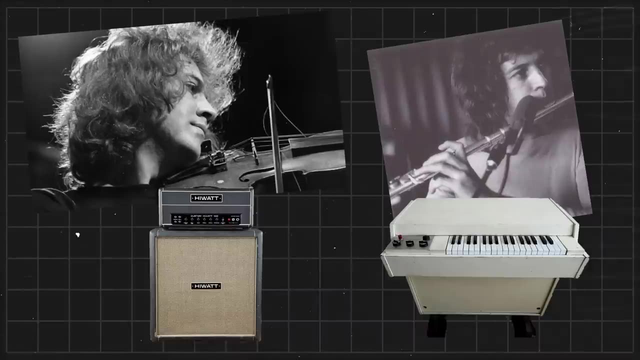 and a viola and a flute, also with hi-watt amp and speakers, plus volume fuzz and wah-wah pedals, as well as another Mellotron 400.. Bill Bruthard's setup consisted of a Ludwig kick and snare. 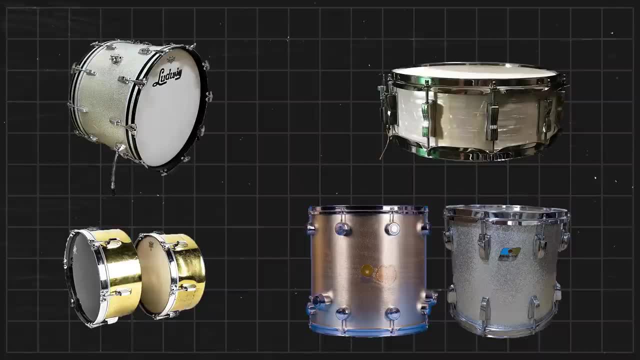 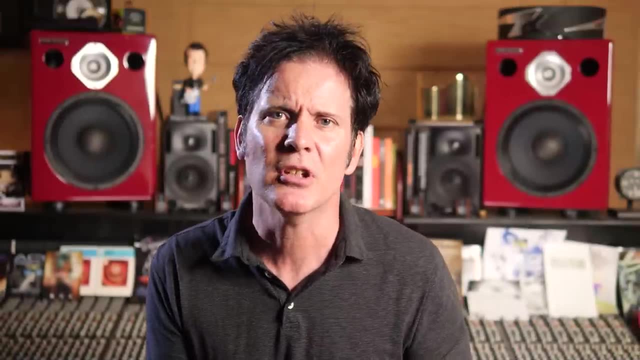 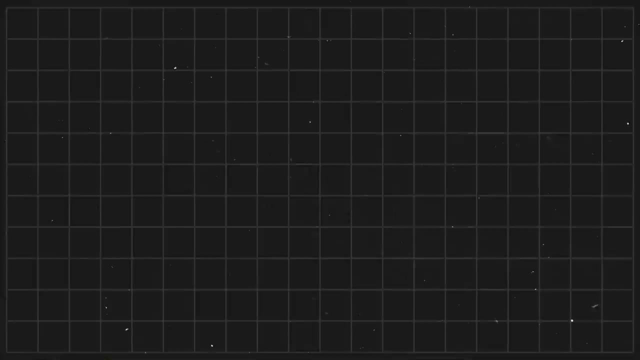 premier timbales, Heymann and Ludwig, toms, pasty cymbals and various other bits and pieces. In January and February of 1973, the Quintet went to Command Studios in London to record its first record, which was self-produced and engineered by Nick Ryan: The resulting album. 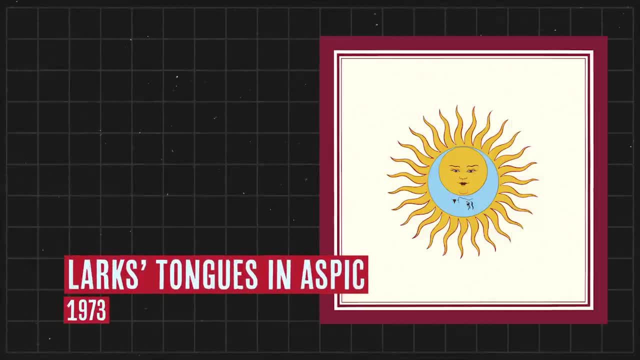 Lark's Tongues in Aspect was spectacular. King Crimson had finally produced an album as good, if not better, than its debut. Bruthard once referred to the band sounding like dissonant shadows on steroids, which makes it more understandable that the band's music went. 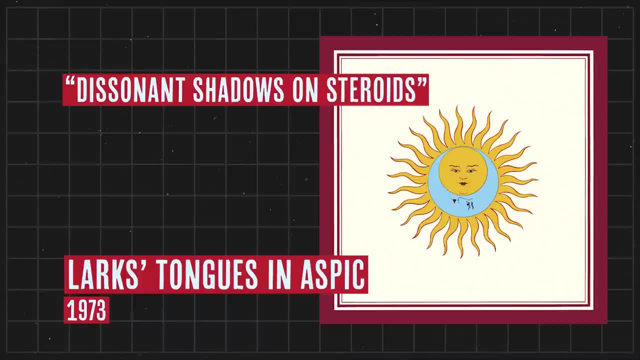 over the heads of some critics. Negative reviews became a commonplace experience for the band. but Lark's Tongues in Aspect has become a commonplace experience for the band. but Lark's Tongues in Aspect has been recognized as one of the greatest rock albums of all time, with one person writing. 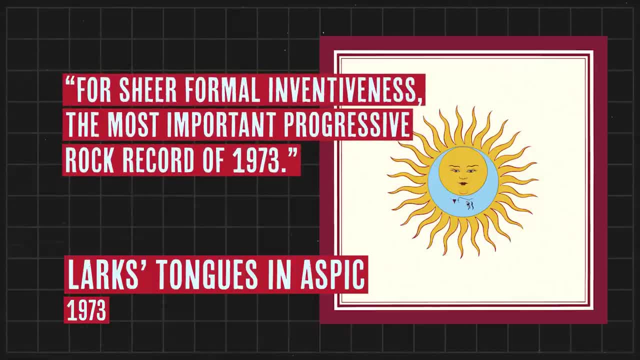 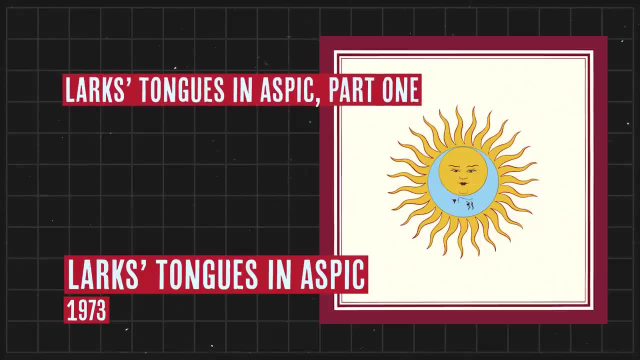 that it was for sheer formal inventiveness, the most important progressive rock record of 1973.. The two title tracks Lark's Tongues in Aspect, Part One and, in particular, Lark's Tongues in Aspect, Part Two, became the blueprint for an abrasive, almost atonal, avant-garde rock style. usually written by Fripp. that has become one of the main characteristics of King Crimson. By contrast, Book of Saturday showed the polar opposite: a tender, gorgeous ballad of the highest quality sung by Whetton During a gig in February of 1973, a gong fell on Muir's foot. 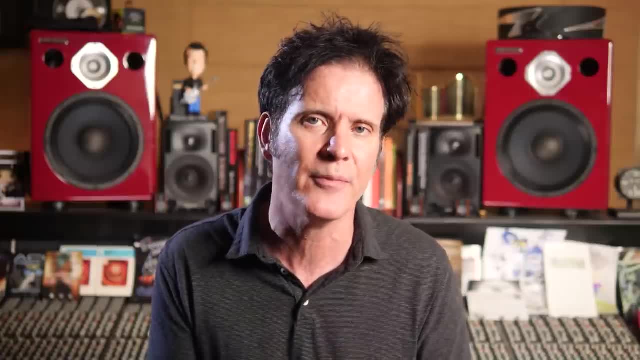 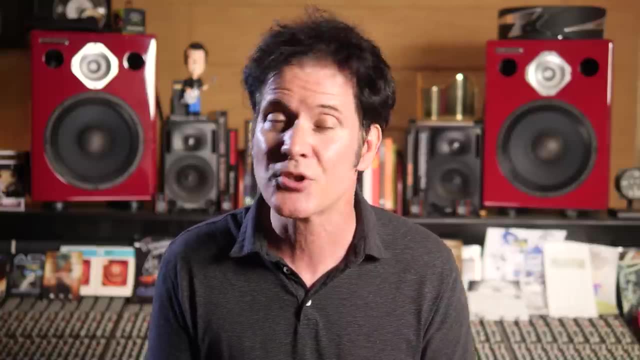 and he was sufficiently injured to be unable to continue to play live. A week after the release of Lark's Tongues in Aspect, Muir left the band and went to live in a Buddhist monastery in Scotland. His influence nevertheless continued to loom large, in particular on Bruford, who said: 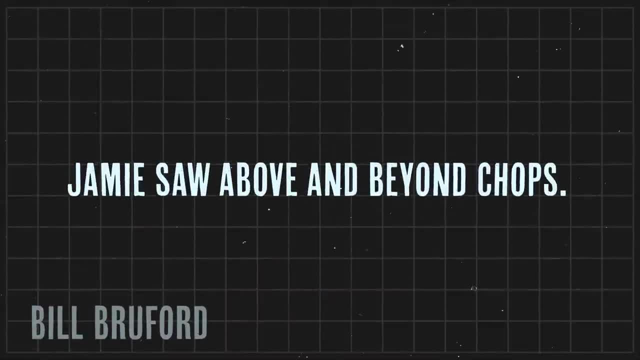 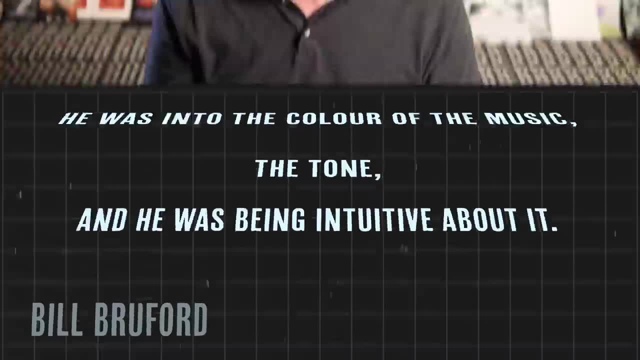 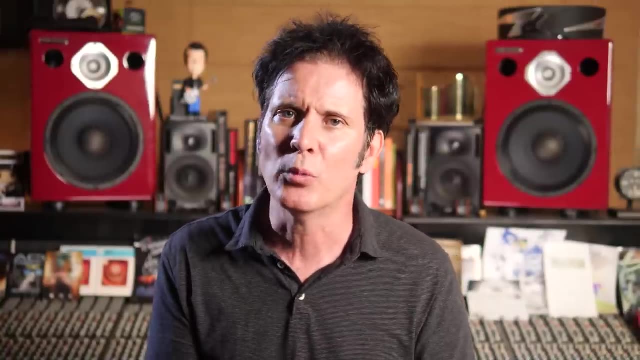 that Muir turned my head totally around. Jamie saw above and beyond chops. He was into the color of the music, the tone, and he was being intuitive about it. Crimson continued touring and flattening audiences, often playing music from Fripp and Eno's No Pussyfooting album while they walked. 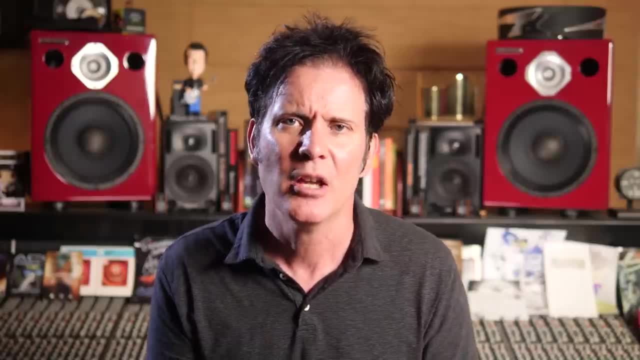 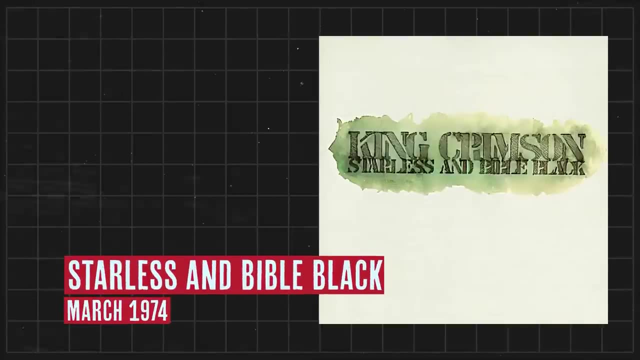 on and off stage. Given the band's spectacular performances, Fripp hit on the idea of basing a new studio album on their live performances. The resulting album, Starless and Bible Black, was released in March of 1974, and is mostly based on live recordings from 1973 in Amsterdam, Zurich and Glasgow. Only two tracks. 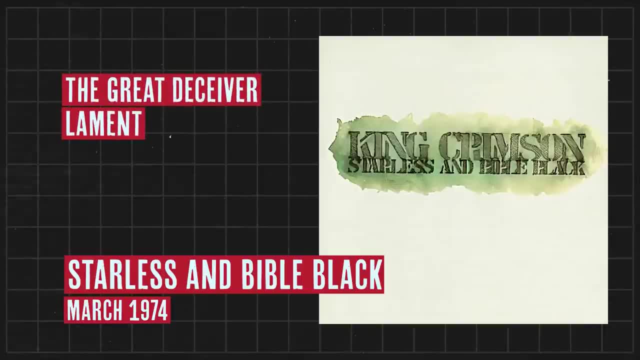 The Great Deceiver and Lament were entirely recorded at Ayr Studios in London. Now it seems the barbies burst. well, you know that The The Barbies burst. well, you know that The Barbies burst. well, you know that. 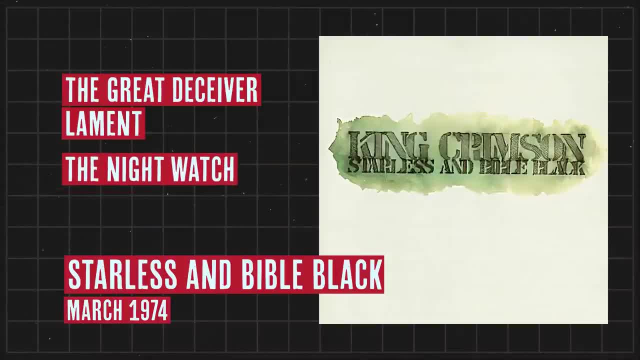 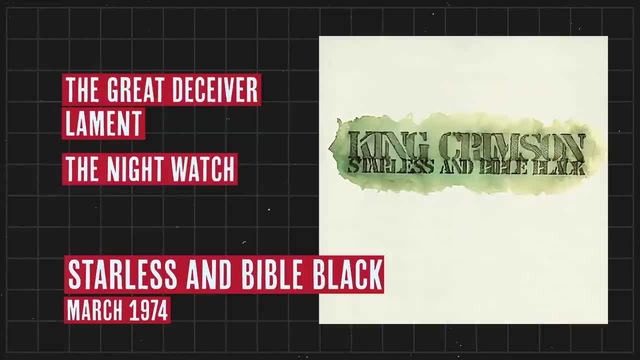 The entire album was edited and mixed at Ayr with George Chiantz engineering. The excellent recording quality of the live recordings meant that many people were not aware that Starless and Bible Black is, at heart, a live album, until Fripp revealed the fact a few years later. 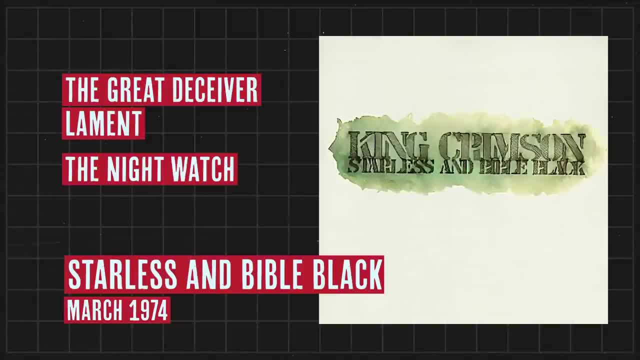 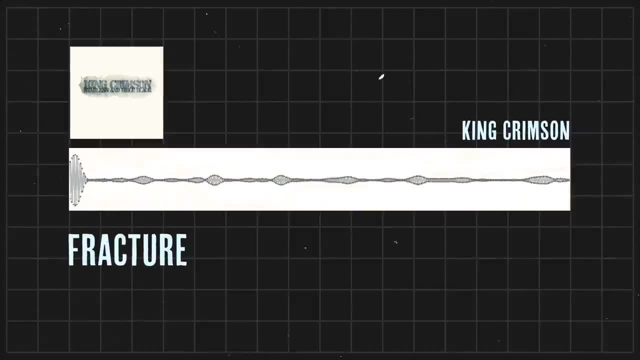 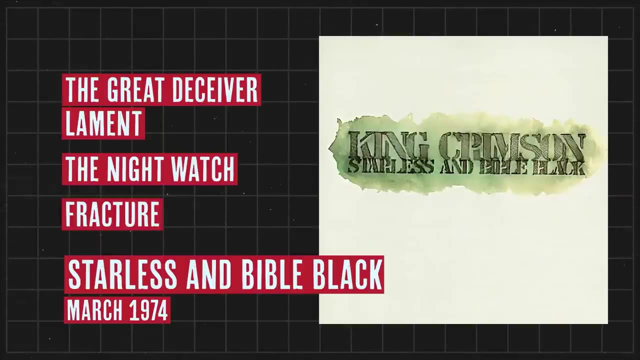 The music on Starless and Bible Black is a development of Lark's Tongues in Aspect. with Fracture, another piece of abrasive, whole-tone avant-garde metal, And The Nightwatch, another sumptuous ballad with an exquisite guitar solo by Fripp. 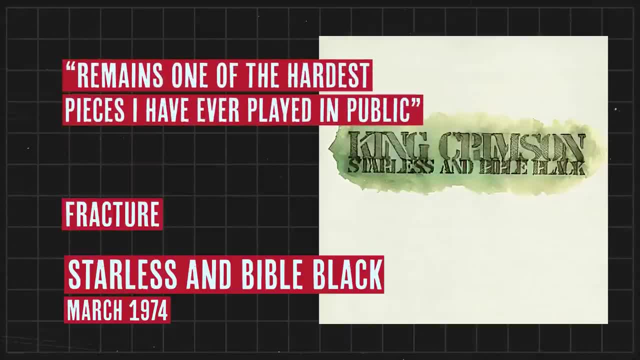 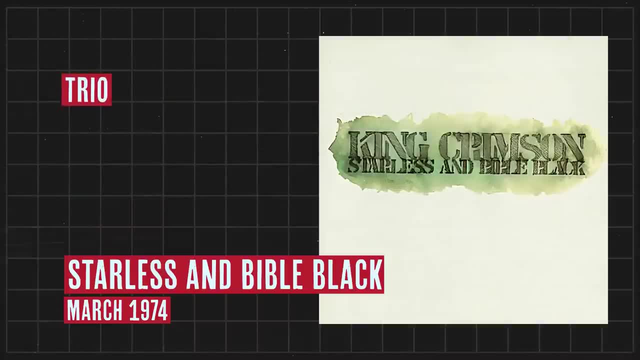 He commented many years later that Fracture remains one of the hardest pieces I have ever played in public. The Pastoral Trio is an unusual live improvisation with Wetten on bass, Cross on viola and Fripp on flute-melotron and Bruford. 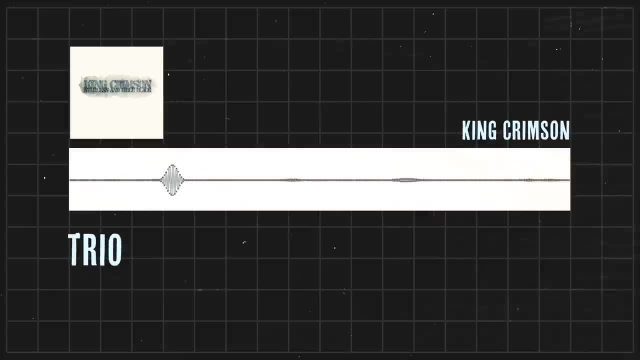 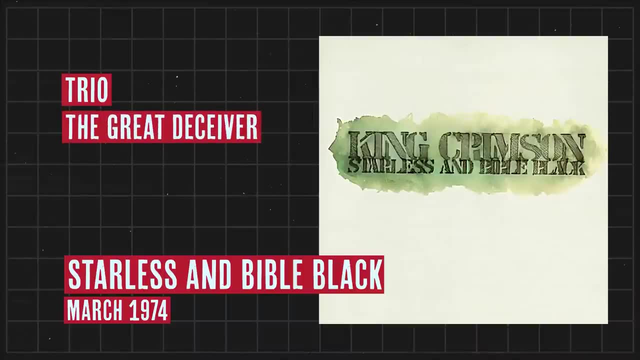 sitting with his hands across his chest, not playing. The Great Deceiver has a guitar riff that is vaguely influenced by blues and sounds like an attempt to create a single, or at least something that could be played by an adventurous radio. DJ Starless and Bible Black was by any intelligent musical yardstick. 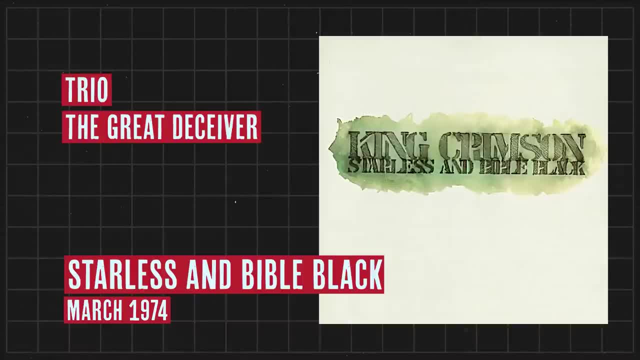 a hugely successful achievement, And the fact that it was mostly recorded live illustrates a point that Fripp has often made, which is that King Crimson is a live band first and a studio band second. He has said Performance is where the juice resides. 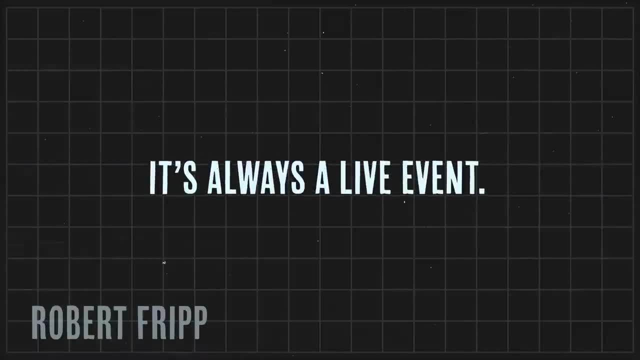 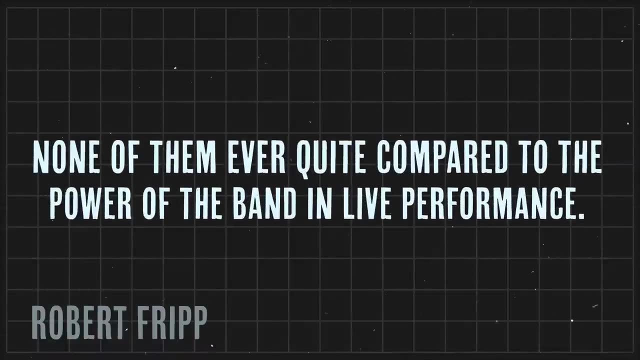 King Crimson has always been a hot date. It's always a live event And however good some of the albums have been, none of them quite compare to the power of the band in live performance. All good things come to an end, and around the time of the release of Starless and Bible Black, 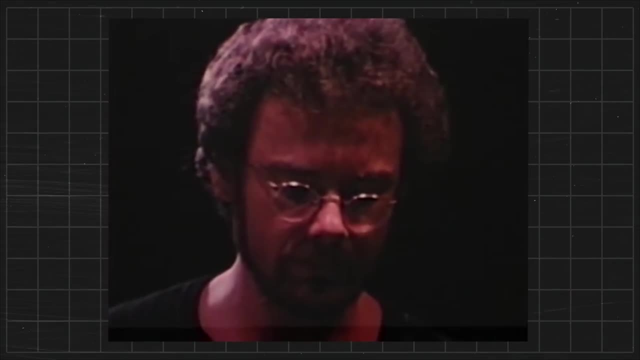 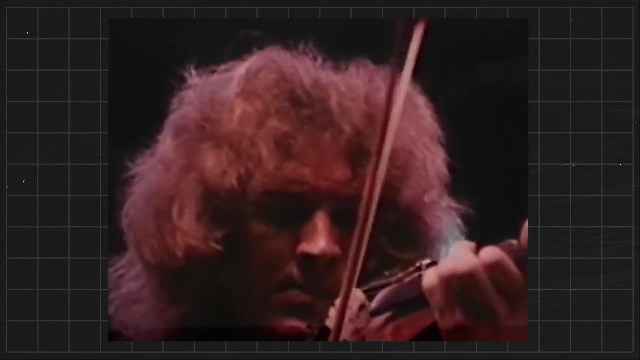 cracks were beginning to show in the third incarnation of King Crimson as well. Violinist David Cross Cross expressed his frustration with losing the on-stage loudness battle with other instruments and complained that most of our improvisations come out of horror and panic. 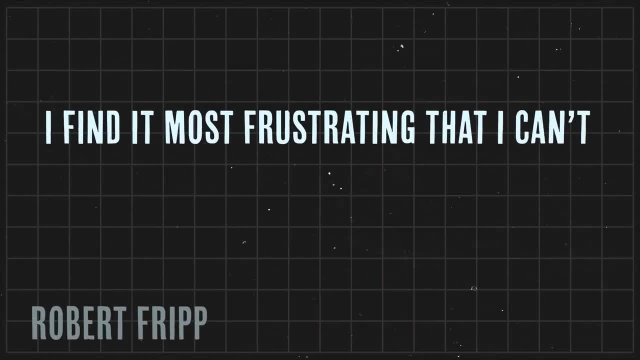 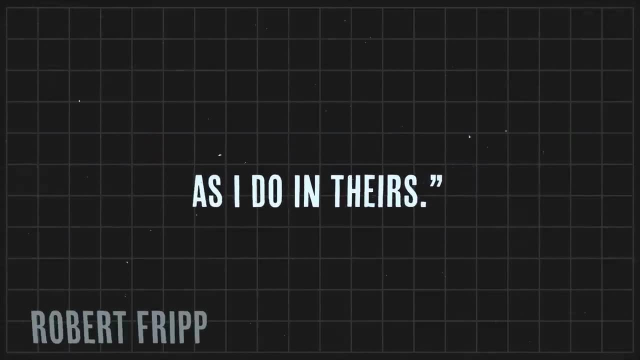 Fripp also had mixed feelings and stated in an interview: I find it most frustrating that I can't make the other players in the band take as much interest in my playing as I do in theirs. After some chaotic concerts at the end of 1973 in Italy, 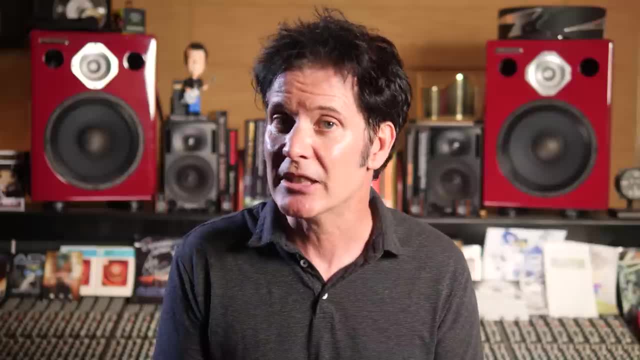 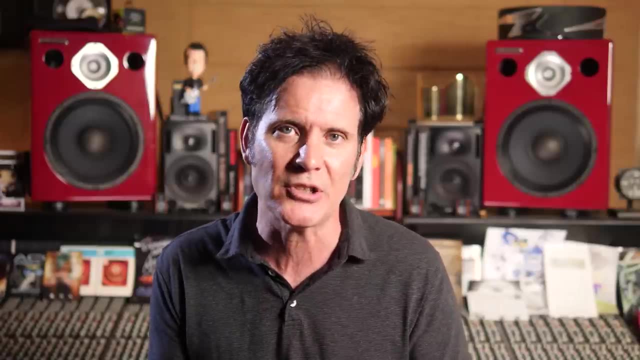 that were marred by violence and drug abuse. he became increasingly dissatisfied with rock and roll live performance. in general, Fripp remarked that the band's approach had become brutal and uncreative. We battered the audience for 40 minutes to make enough room for 10 minutes of experimenting. 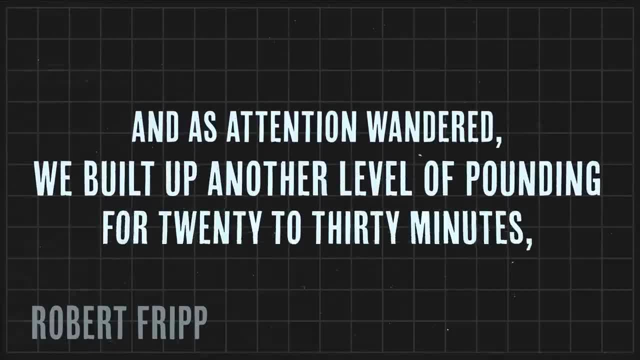 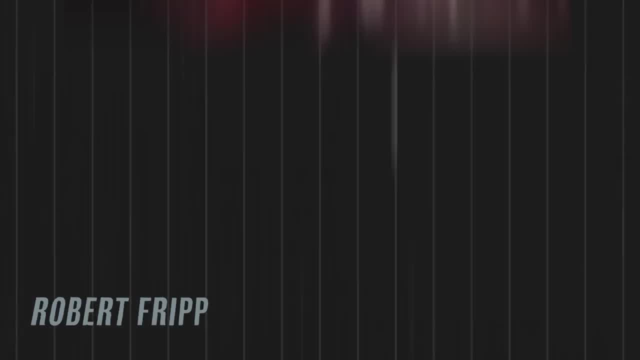 And as attention wandered we built up another level of pounding for 20 to 30 minutes, so the pulped crowd felt it had its money's value and would go home happy. King Crimson Mark III played its last concert on July 1, 1974, in Central Park in New York. 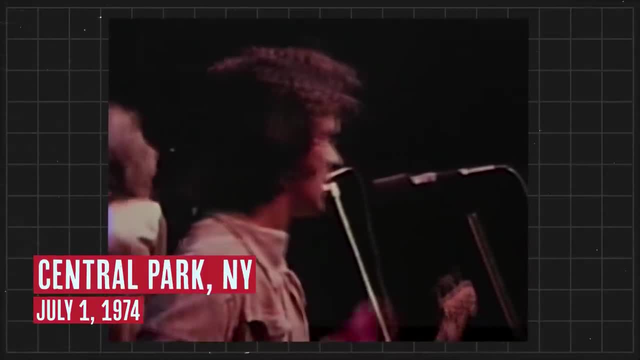 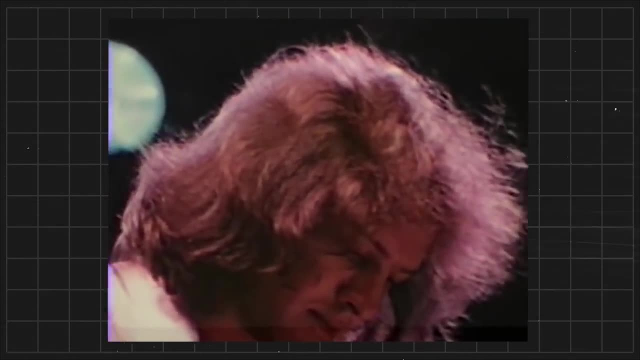 days after the release of Starless and Bible Black, After the live recordings for another live album, USA. she was not released until 1975.. David Cross left the band immediately after the tour and on July 8, 1974,. 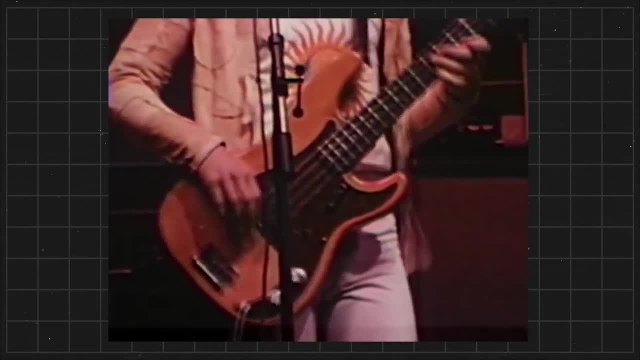 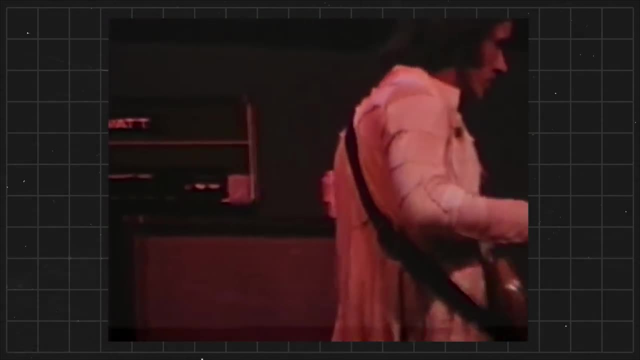 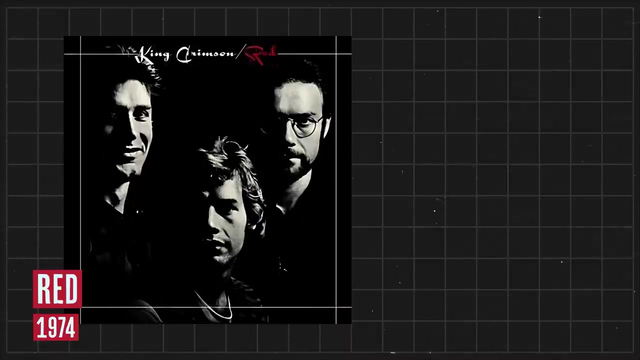 Fripp, Whetton and Bruford went to Olympic Studio II in London to record another album with engineer George Chance, again at the controls. Despite, or perhaps because of, the tense circumstances, the resulting album Red became arguably the highlight and defining achievement of King Crimson's entire career. 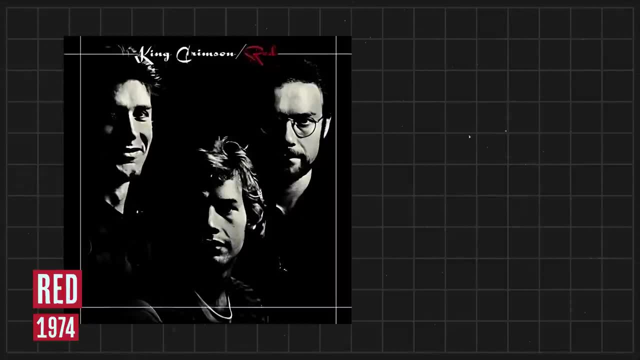 Similar to on Starless and Bible Black. one live track was included, Providence, recorded on June 30, 1974 in Rhode Island with David Cross. The other four tracks were all recorded at Olympic Studios, which makes Fripp's own assessment all the more remarkable. He called King Crimson III. 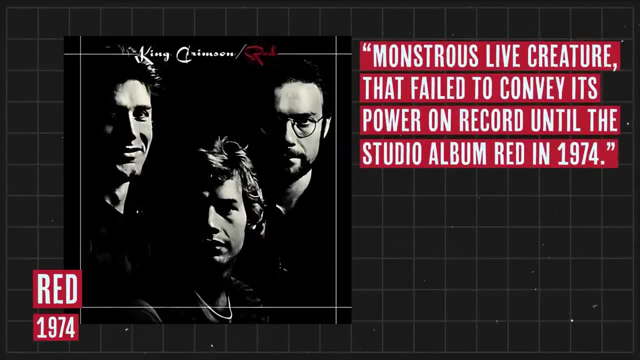 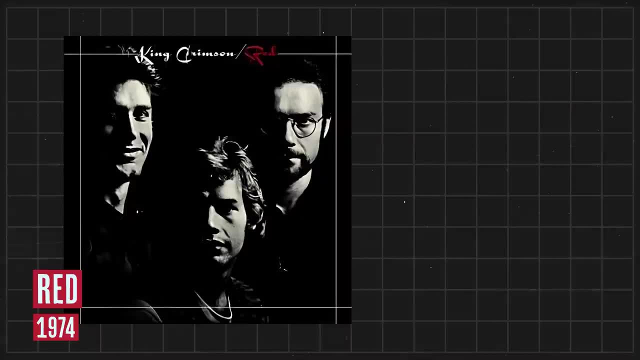 a monstrous live creature that failed to convey its power on record until the studio album Red in 1974.. He has communicated on several occasions that Red is one of the few, if only studio albums that really conveys the power of King Crimson's music. He has also said that King Crimson has 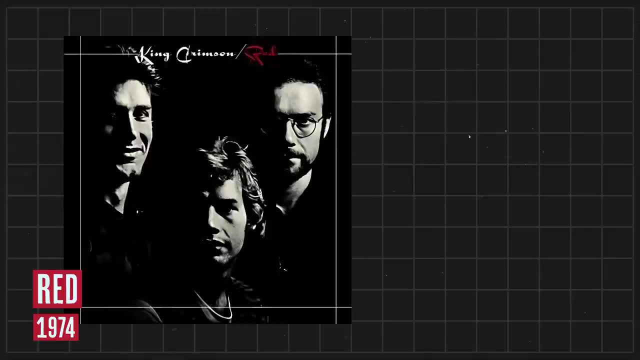 been a great influence on Red's opening musical track and that it is one of the most popular community shows of the year. The immense power of the band is immediately and fully realized on Red's opening track. The instrumental is based on a whole-tone scale with the guitar and bass. 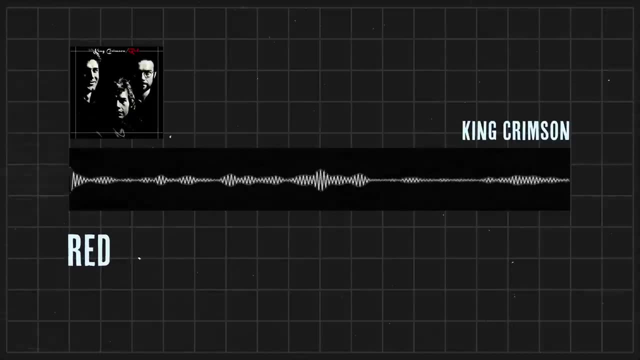 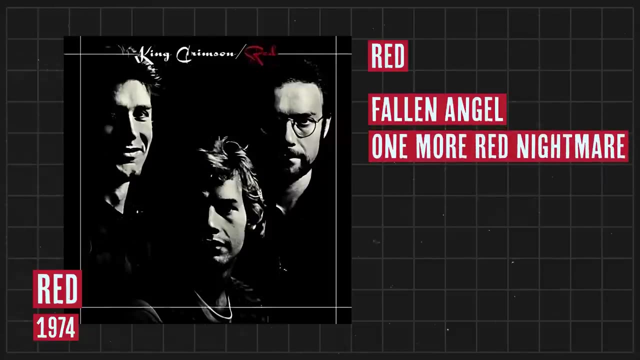 playing a tritone apart, Fallen Angel and One More Red Nightmare are more traditional, melodic and feature the reintroduction of wind instruments like saxophone, cornet and oboe. However, However, the high point of the album and arguably of King Crimson's entire oeuvre, 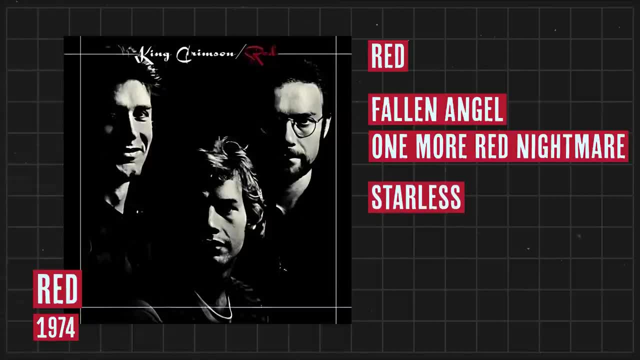 is the 12-minute-long closing track Starless, Featuring Ian MacDonald and Mel Collins on saxophones and Julian Lloyd Webber on cello. the track starts with a melancholy ballad in G minor in the vein of Book of Saturday. 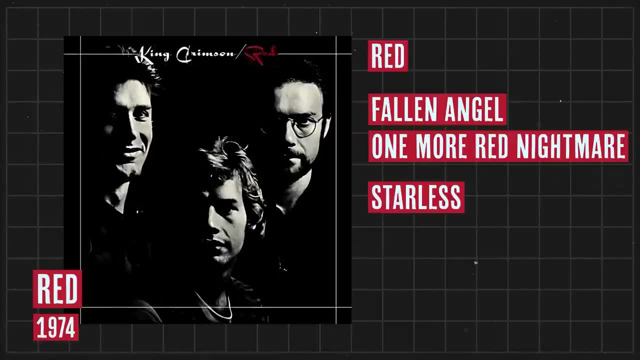 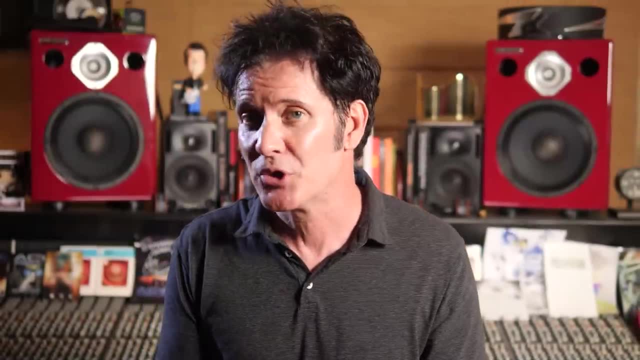 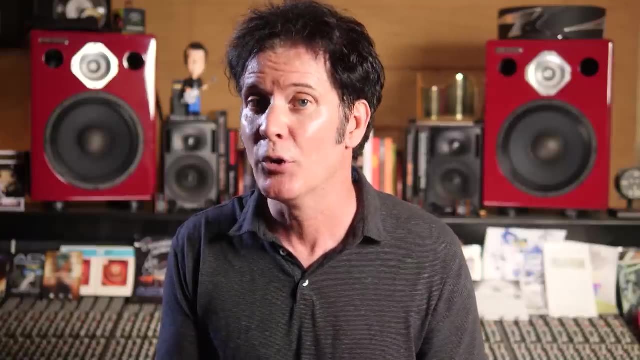 and The Night Watch, featuring a mellotron and a majestic instrumental theme played by Fripp. The vocal melody and the chords were written by Wetton. The ballad transitions into an instrumental in 13-8, that starts quietly and gradually, builds in intensity and culminates in a wild improvisation, first in 13-8, then 4-4.. 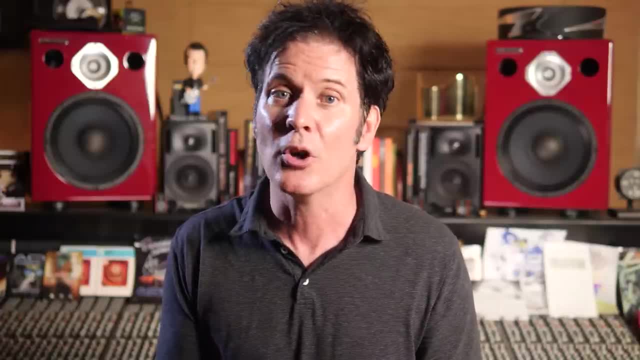 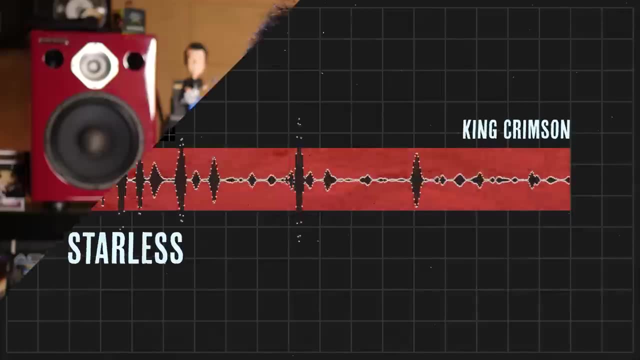 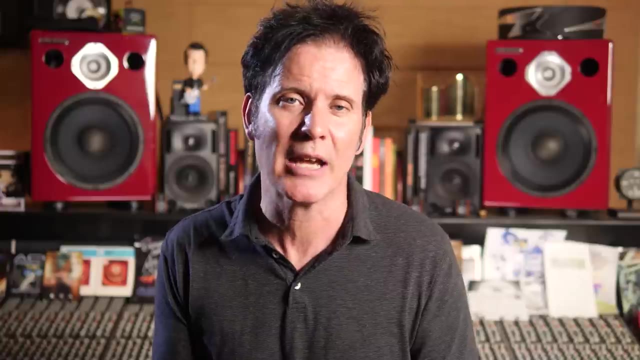 At the end there is a return to the earlier majestic theme played on saxophone. this time, The track is a masterpiece of melodic inventiveness, suspense and gradually builds up to an astonishing climax. Red has been called Progressive Rock's finest hour, and one could say that King Crimson 3. 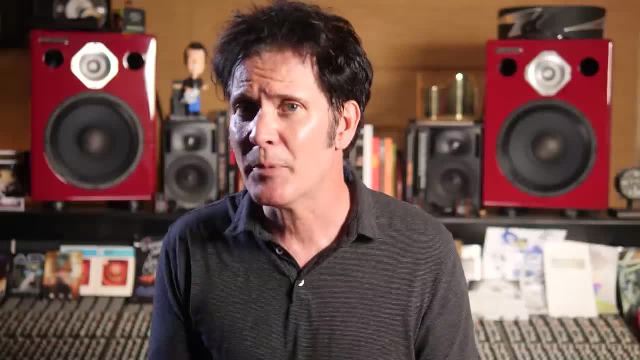 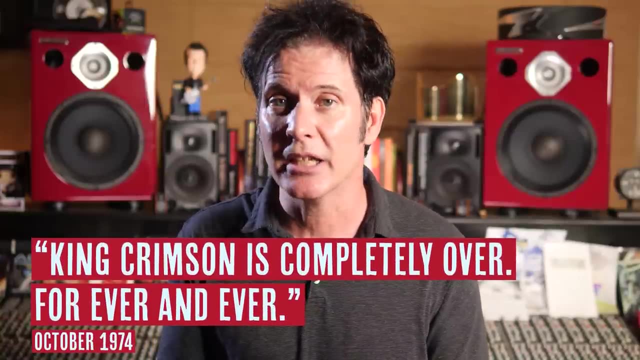 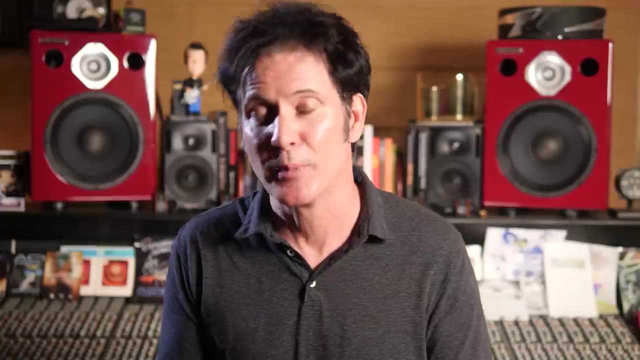 had fulfilled its destiny and this made the end of the band inevitable. It was announced before the release of Red in October. In an interview, Fripp said King Crimson is completely over forever and ever. Fripp took a three-and-a-half year hiatus from the music industry for personal and spiritual. 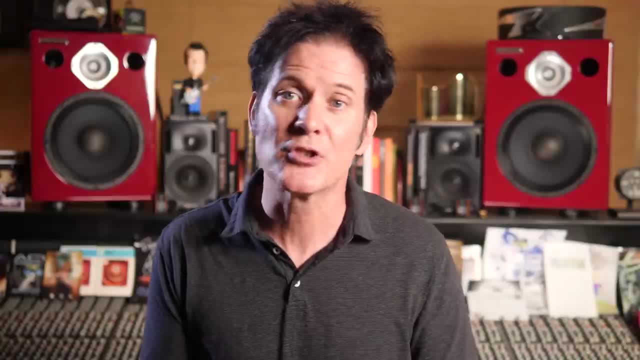 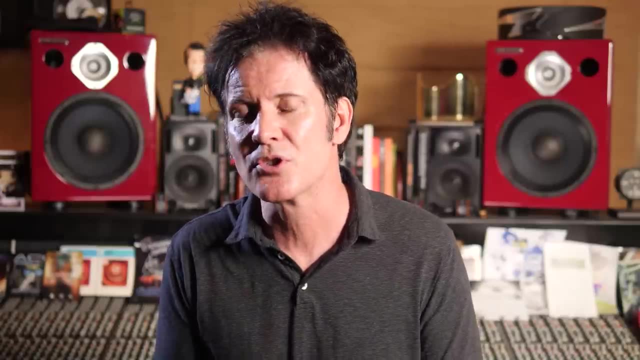 reasons In 1977, he was eventually dragged back to life as a professional musician by David Bowie Gabriel, on whose albums he played most famously and iconically on Bowie's song Heroes. Fripp's DGM Live label has, over the years, released a significant number of boxed sets. 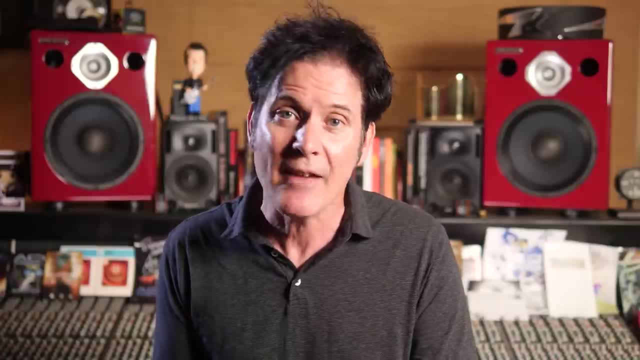 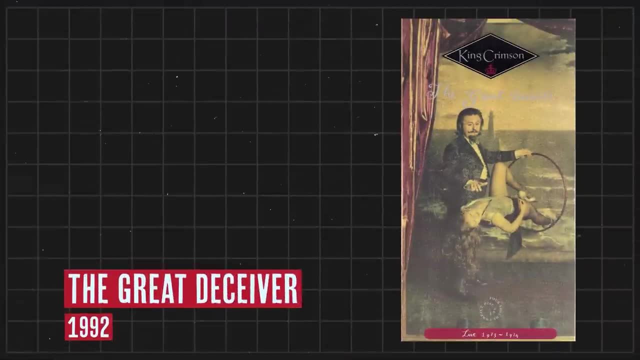 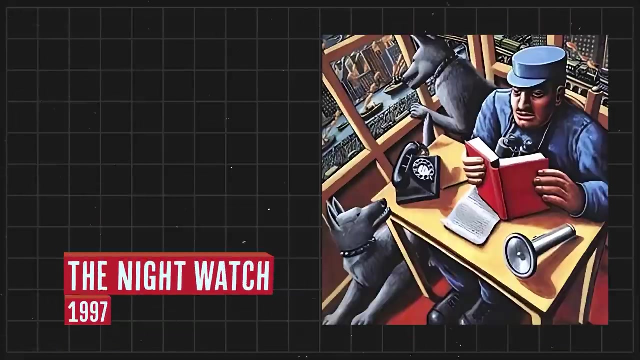 with more material from the 1968-74 era, with a heavy emphasis on the 1972-74 band. This started with the release of a four-CD boxed set, The Great Deceiver in 1992, which contained live performances from 73 and 74, and then The Night Watch in 1997.. 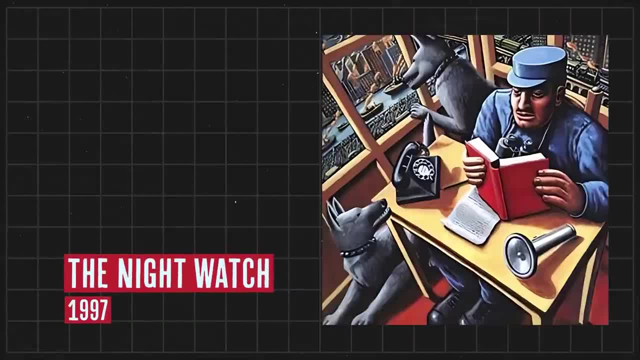 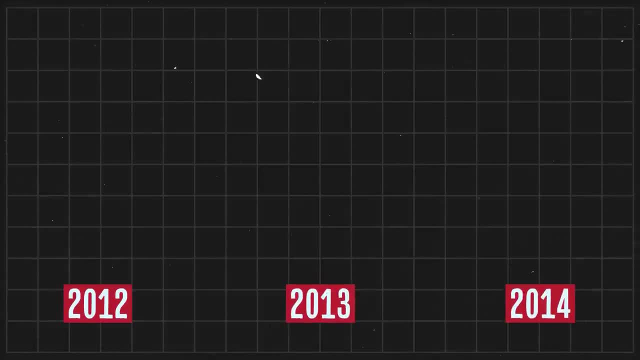 With the entire Amsterdam concert, from which much of Starless and Bible Black was taken. In 2012,, 2013, and 2014,, DMG released three 40th Anniversary Edition boxed sets that covered the 1972-74 incarnation of King Crimson, containing a whopping 64 discs in total. 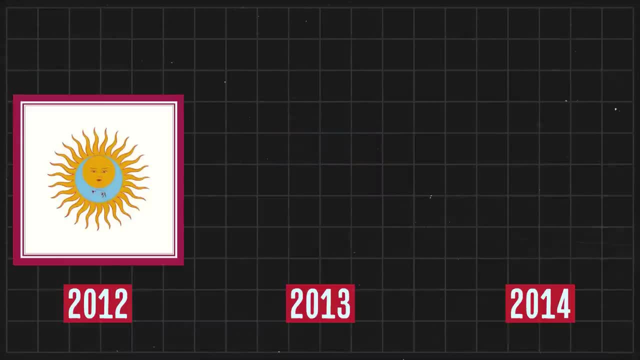 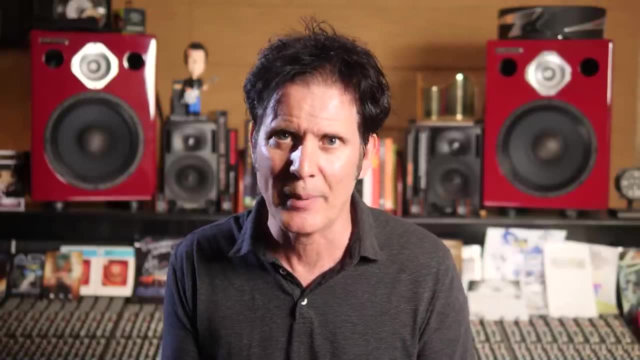 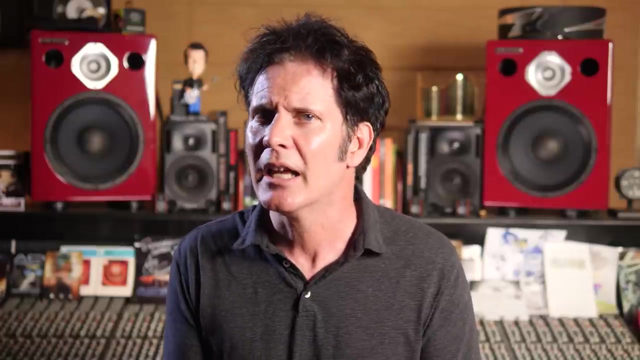 The boxed sets were called Lark's Tongues in Aspic, Starless and The Road to Red. From 21st Century Schizoid Man- the first track on the band's first album, released in 1969, to Starless. the last track on Red, released in 1974, encompasses many remarkable 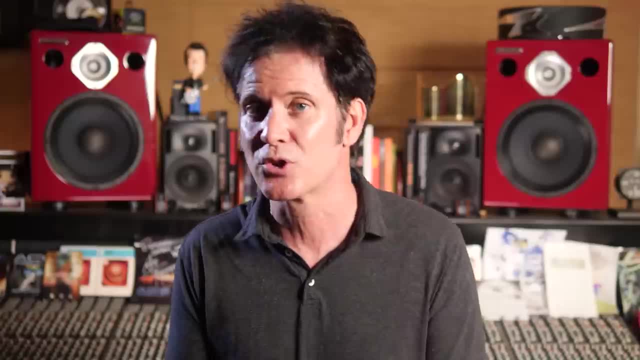 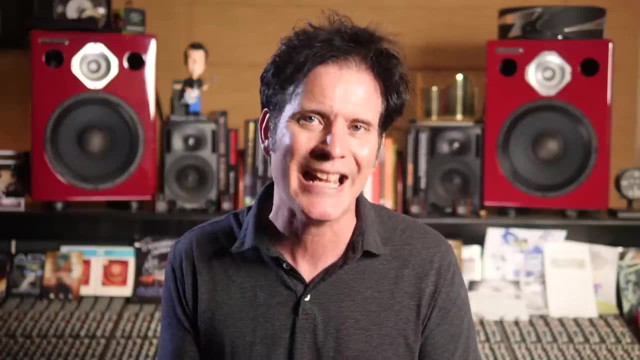 creative achievements that change music and continue to be a strong influence on music today. Despite Fripp's assertions in 1974, the story of King Crimson did not end that year. In 1981, he revived King Crimson again with a completely different musical approach. 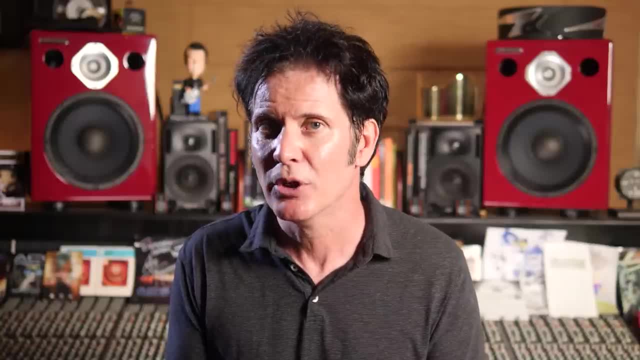 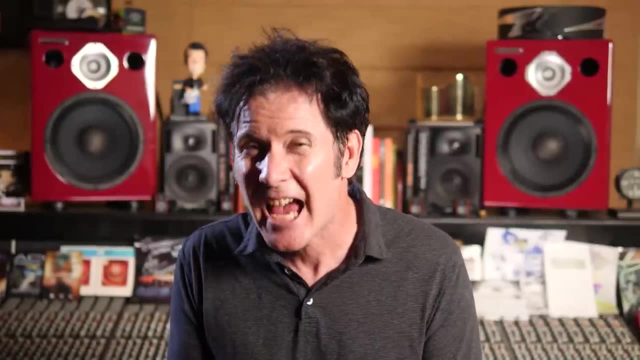 He was Toufford bassist Tony Levin and guitarist Adrian Ballou. We'll look at that and what came after in the next video. Thank you ever so much for watching. I cannot overstate how important King Crimson are.